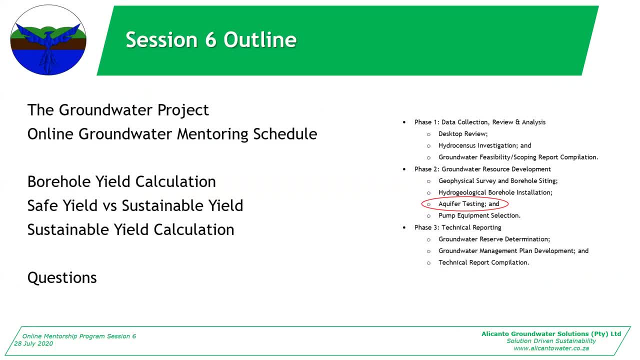 In this session we're going to go through the sustainable yield determination, which is part of your aquifer testing, but it's more also part of your licensing and the overall processing for a borehole. Yeah, we'll go through just the groundwater project, just to remind you guys to check that out. 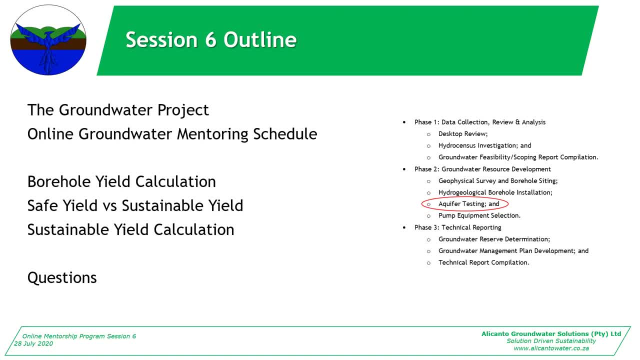 And then the online schedule, just to remind you guys where we want to go from here, And then the three main things we're going to do. The three main sections we'll go through tonight is the borehole yield calculation, safe yield versus sustainable yield, and then the sustainable yield calculation. 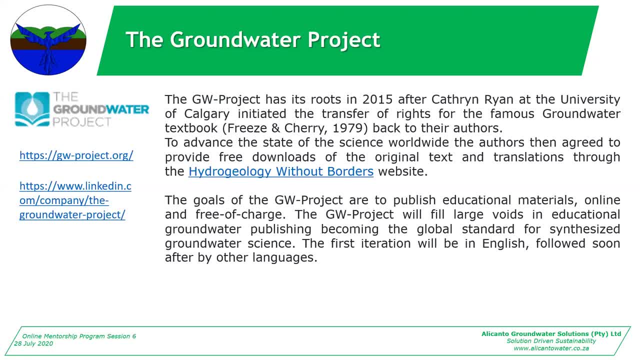 Okay, so Groundwater Project started with the Hydrogeology Without Borders website, where they're trying to share and publish groundwater educational materials free of charge. I see today on LinkedIn that they're going to release a new sort of proprietary book or unique book to Groundwater Project on the groundwater cycle. 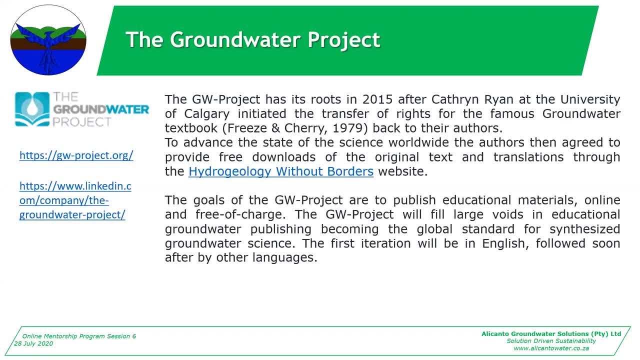 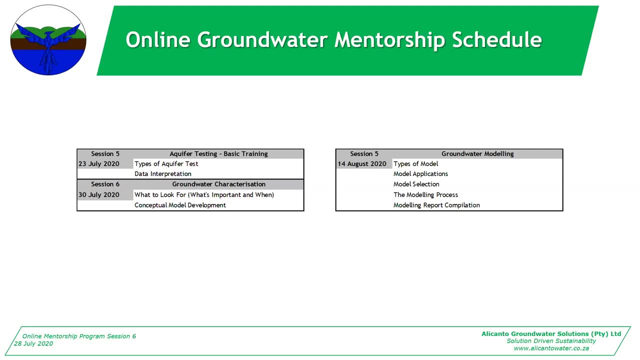 which will be worth looking at. If you guys haven't followed them already on social media, I suggest you do that and register on their websites as well. It's a really worthwhile program that they're running. In terms of the schedule, today we're doing the. 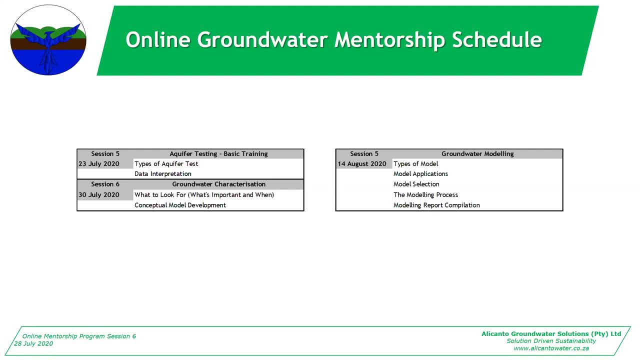 the aquifer testing we're extending on the sustainable yield, which we didn't do last time. So session six on this slide will become session seven, which will be on Thursday, And that'll be the groundwater characterization- what to look for. 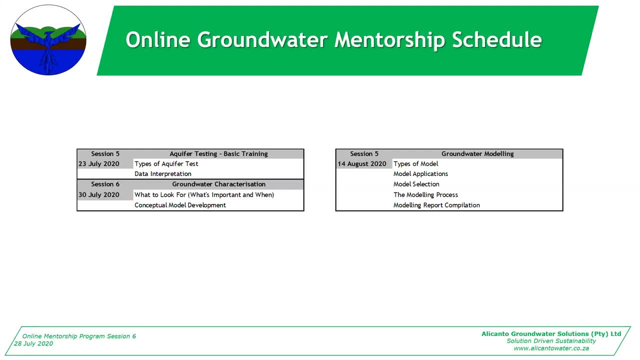 what's important and when it's important. Yeah, that's in terms of what kind of project you're doing, And then we'll focus on the conceptual model development, which is quite an important part of any groundwater study. Yeah, whether it's a. 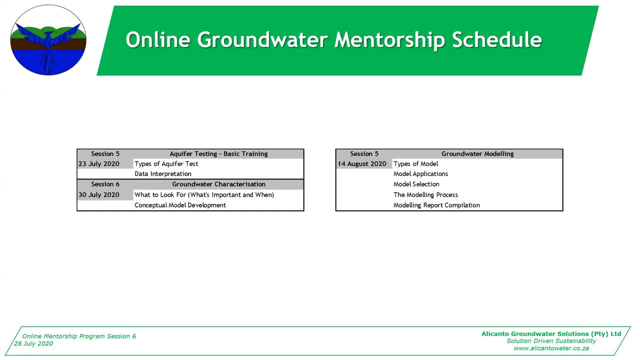 a resource development project or a mining project or any kind of groundwater project. the conceptual model is is very important for your results. Then in August we'll focus on groundwater modeling. We'll go through it at a high level. types of the models we use. 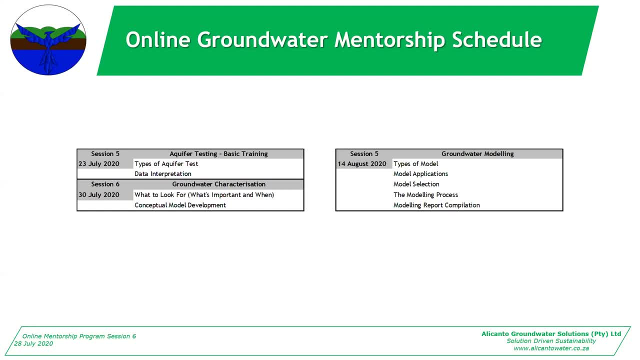 the model applications that we do typically: selecting your model, what sort of parameters you need to consider, then the modeling process and then compiling your modeling report. Is there any suggestions for another session after groundwater modeling that you guys can can sort of think of, that you would like to see and be a bit exposed to? 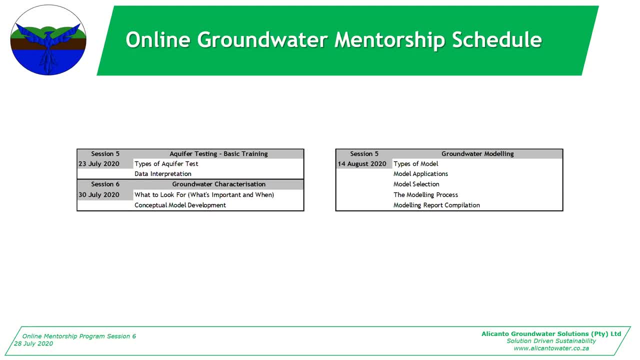 Matthew, can we do? can we do something related to mines? Like you know, the mine water decanting, the whole process, ground water related in a mine, if that's possible, Yeah, Yeah, And I think Lizelle can also contribute to that one. 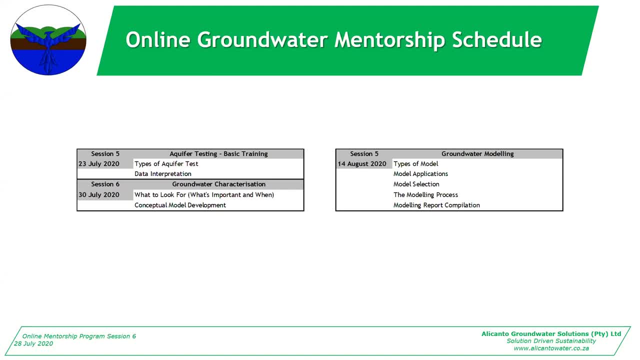 you know, with your masters. Lizelle, Yes, I did pit lakes on coal mines which is essentially decant from open cast operations. So, yeah, I know a bit about the chemistry, Yeah, And so on. Yeah, Well then let's make that sort of session eight or whatever it works out, to be able to mine hydrogeology. 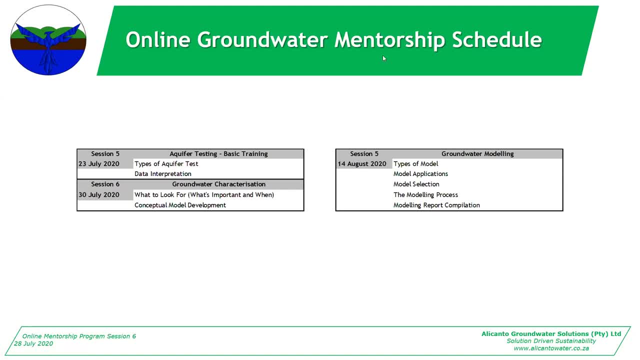 Okay, Thanks. So any other suggestions on what you want to be exposed to guys? Hi, Matthew, Maybe groundwater monitoring and management? Okay, In terms of what exactly like the design of the network or the execution, Like everything, Because I haven't really been exposed to the groundwater monitoring part of a hydrogeology. 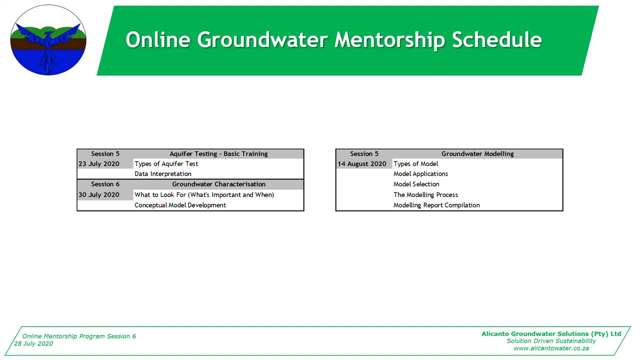 Okay, Okay, Now I'll give it some thoughts. Yeah, So monitoring, monitoring and management, Okay, Yes, Okay, Cool, Anybody else? Matthew, Hey, Victor, I just want to sort of like just a suggestion that when you do the modeling, 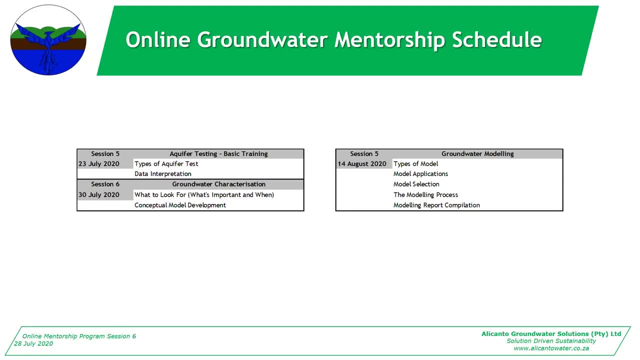 can we also sort of like have a scenario where we go and collect data and come back with it okay, and come back with it in comparated to the model software and then sort of like get a result, maybe in sort of like a situation where we have groundwater? 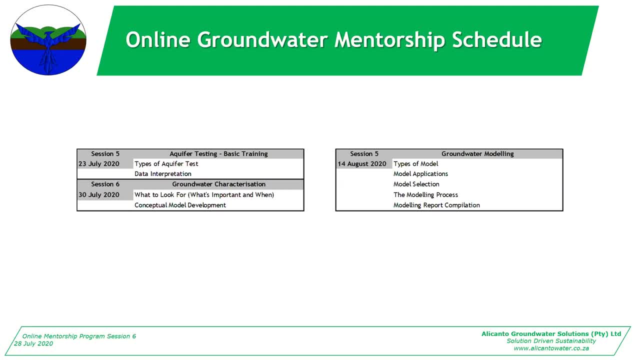 surface water interaction, or rather modelling about contamination, blue movement. It's very difficult, Victor, to do that kind of thing because modelling is such a complicated sphere. I can give all of you guys the same question and the same data sets, and you could give me 10. 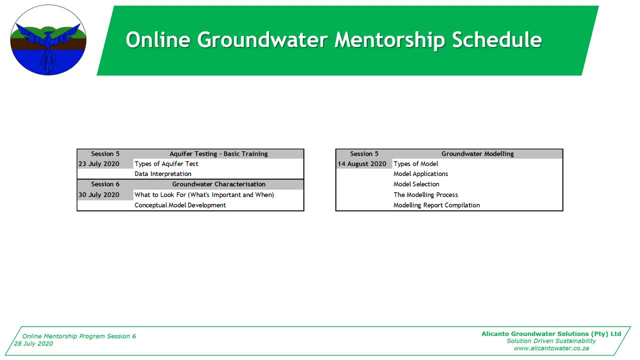 different models and none of you could be wrong. so I think let's look at it on Thursday- and I do want to get back to the exposure side- and then if you guys have specific questions, we can deal with that. but modelling is a it's a complicated thing, Victor. 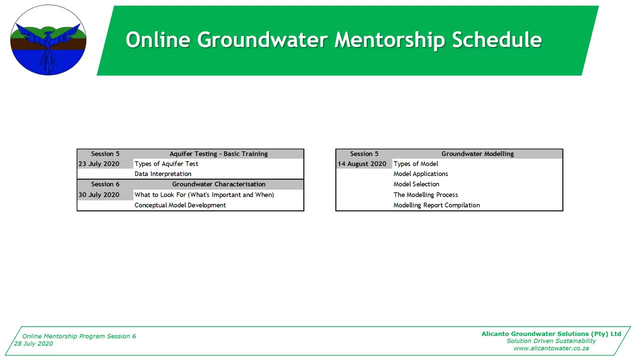 so it can end up taking a lot of time. Alright, alright, Matthew, Have you done modelling before? Victor, Yeah, I'm just exposed and, like we have your mod flow, I'm just a bit familiar with mod flow, so, yeah, Okay, Yeah, look, we'll go through it. 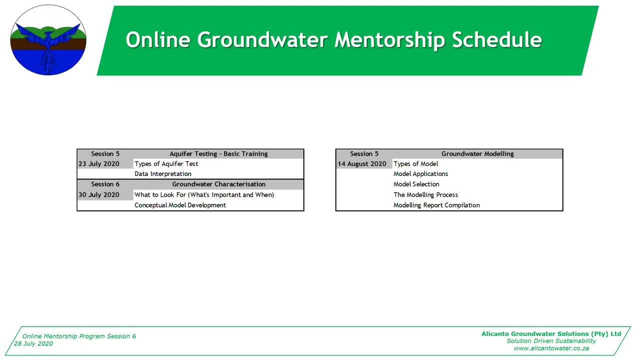 on Thursday and we'll see what happens, what comes out of it. but you know, for now, I think let's, let's just keep at a higher level, because modelling is not for everyone and you don't have to worry about becoming a modeller. you know what I mean. if you don't get it, 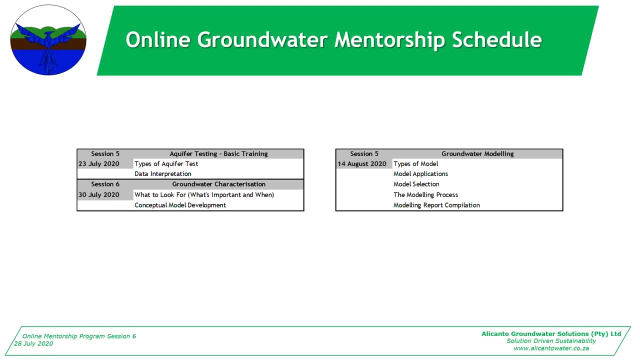 or you don't like it, then it's not the end of the world. Okay, we got a suggestion from Antonia just to focus on hydrogeology and underground mines and tunnels. We'll do a section on that later on in the chat. We've got a discussion on that as well. 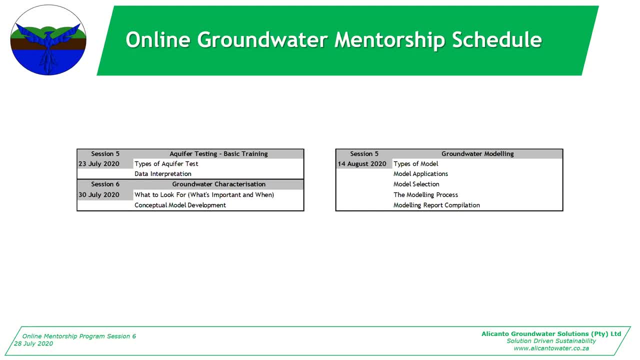 because that's quite a quite an interesting one. Okay, so that takes us up to session 10. then Any other suggestions, Rachel? Any suggestions? Sorry, I was just unmute you. I'll think about it and let you know This is my first session doing so. 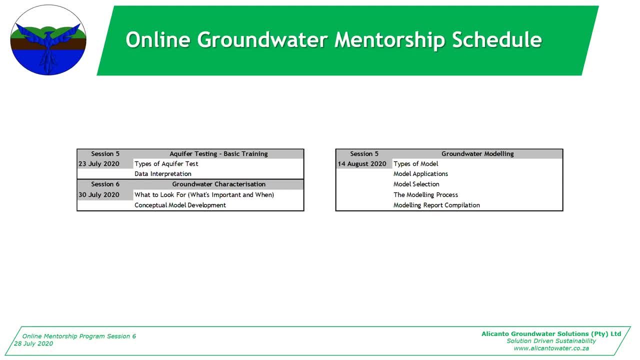 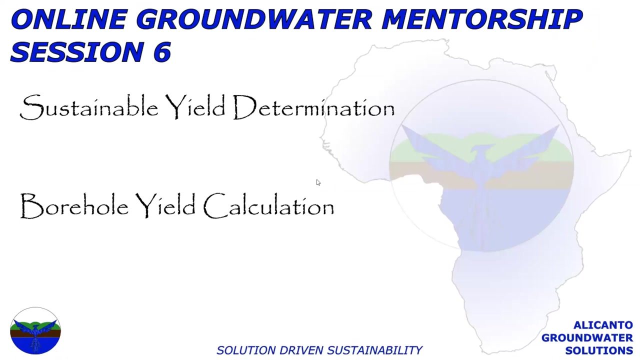 Welcome. I hope it's. I hope it's useful, Thank you, okay, guys, I think let's carry on then. if anybody has something, you can just stop me, but we'll carry on, okay. so first step we're gonna do is the borehole yield calculation, which is from your pump test data. so that's, I've done my pump test. 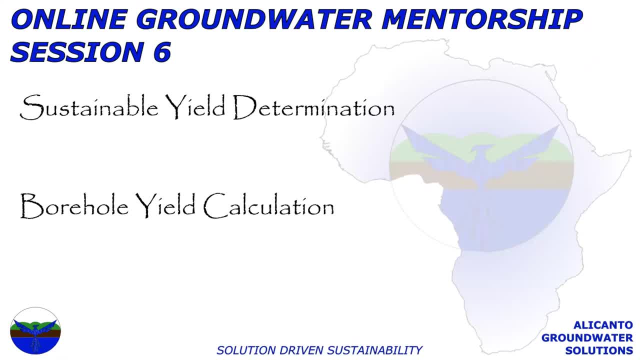 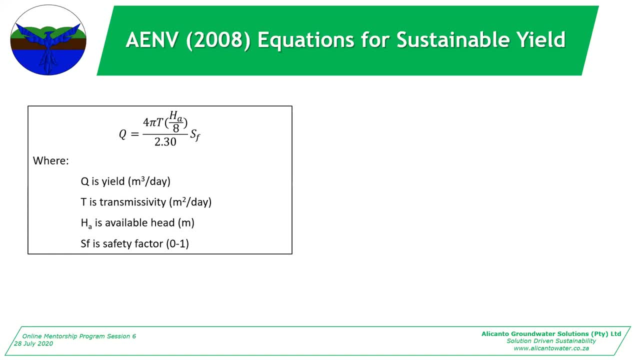 and I want to determine what recommended pump yield I should use for the borehole. so there are equations for sustainable yield by the ae NV. these are quick and dirty calculations. yeah, the first one is your yield. Q is for power transmissivity, your available head and a safety. 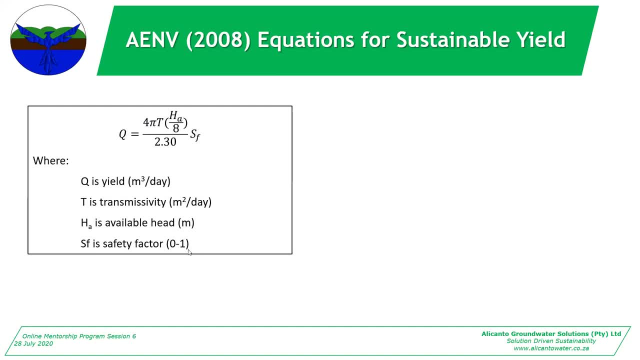 factor between 0 and 1. so think of this as a percentage. so make it point 1 like a 10% safety factor. it'll take you to the next step. so that's the first step and then the second step is the third step. so it's very simple. you just take this number, multiply it by point 1, so you're. 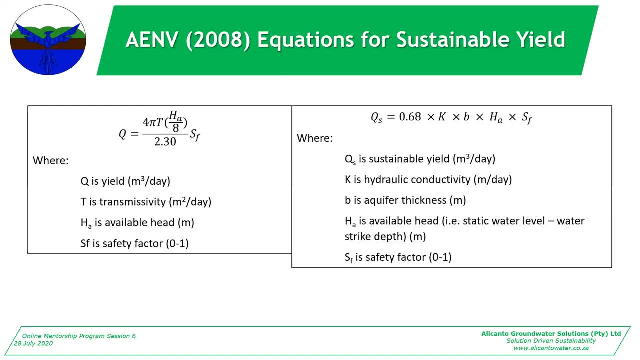 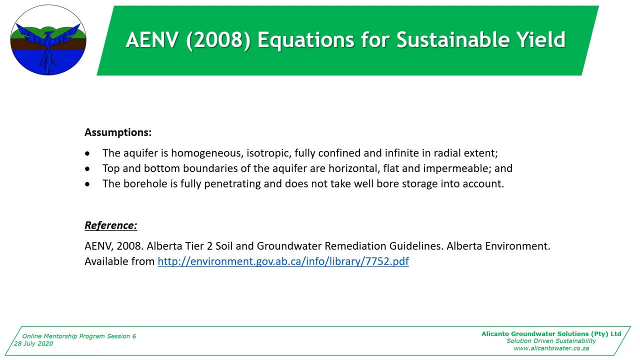 being ultra conservative. and then here's another equation where your sustainable yield is relates to your conductivity multiplied by the aquifer thickness, which gives you transmissivity anyway, multiplied by your available head, your static water level to the water strike depth, and then your safety factor. Yeah, the assumptions on these is that the aquifer is homogeneous, isotropic, fully confined and infinite in radial extent. top and bottom boundaries of the aquifer are horizontal, flat and impermeable, and the borehole is fully penetrating and does not take well-bore storage into account. 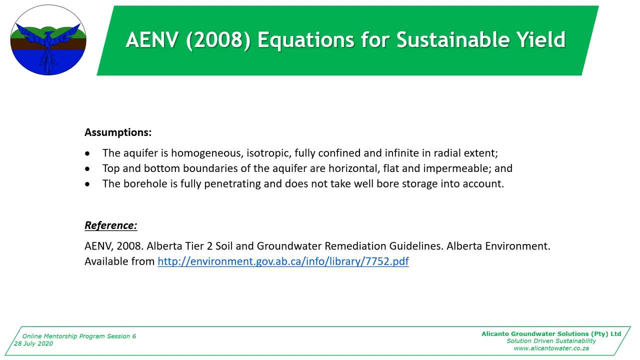 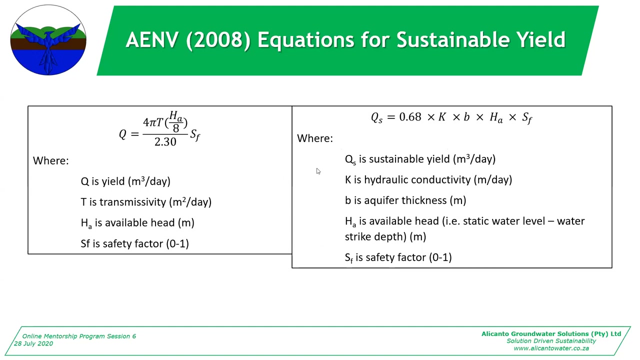 Yeah, does that look familiar to anyone? No, Shocking. These are similar to your Cooper-Jacobs assumptions that we did last week And you can see the 4 pi t is coming out of Cooper-Jacobs t available here, so they're very similar equations. 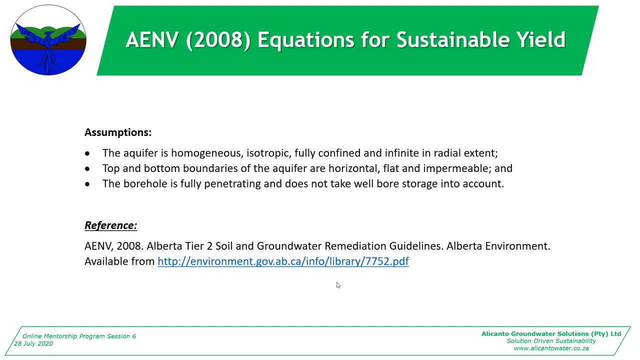 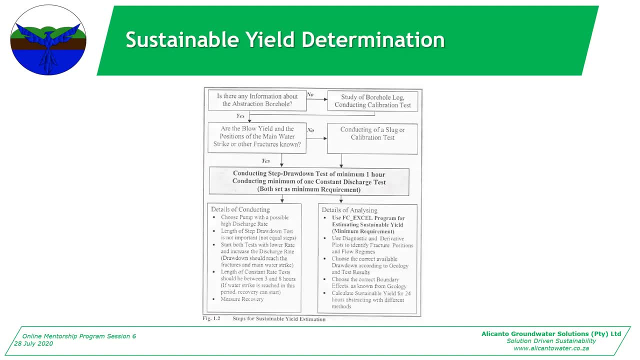 But here is the PDF. I recommend you download it and have a read through it. But this is a quick way to get your sustainable yield And this the typical way we do it in South Africa is through the FC program, which is the flow characterization program from Free State. 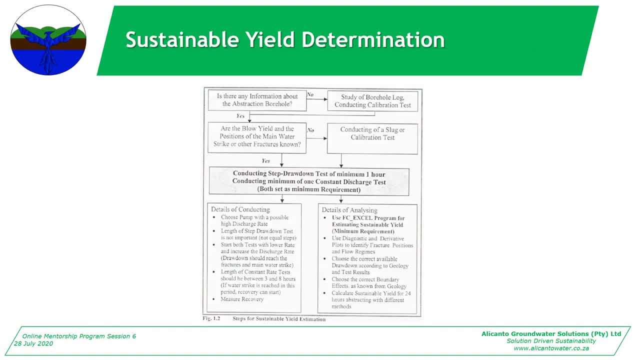 This comes out of the report that Gerrit van Tonde and them wrote about aquifer testing in sustainable yield determination in fractured rock aquifers. So you start off. is there any information about the abstraction borehole? If not, you study the borehole log. then you conduct a calibration test which gives you a rough idea of what's in there. 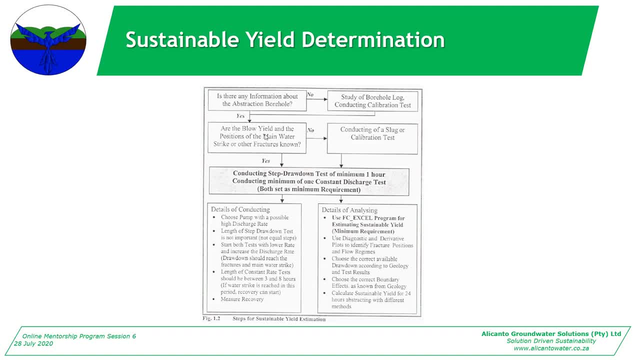 And if there is available information, is that? does that include the blow yield and the main water strike or other water strikes? You remember we spoke about the importance of your hydrogeological log in the previous session, So this helps you with your sustainable yield determination. 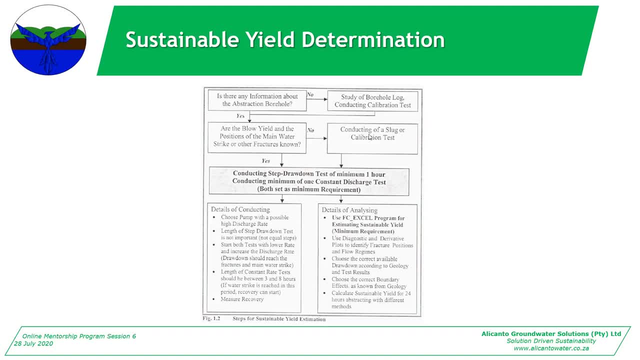 If that's not available, then you need to do a slug test or a calibration test just to get an idea of the order of the magnitude of the aquifer parameters. Once you've done that, you go into your aquifer testing program. 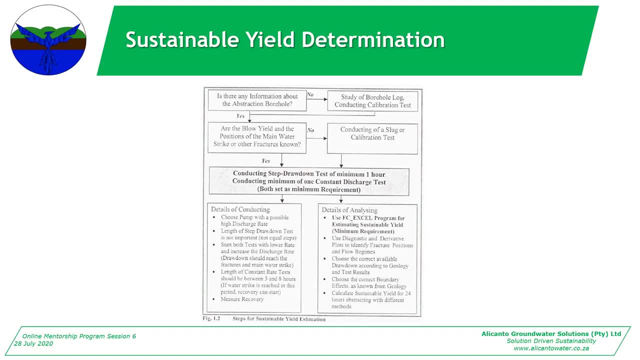 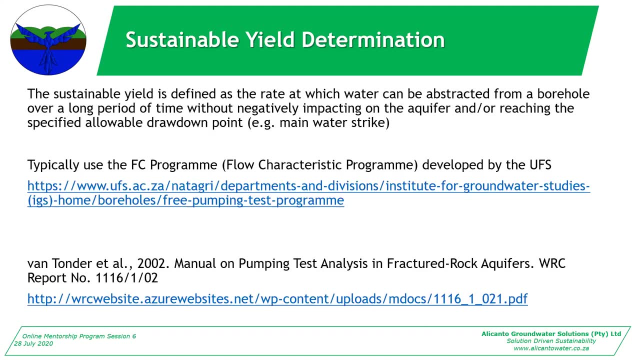 Which consists of your step test and then your constant distraught rate test. Yeah, that's, according to the Science, 10-299 in South Africa. Yeah, so the sustainable yield is defined as the rate at which water can be abstracted from a borehole over a long period of time without negatively impacting on the aquifer and or reaching the specified allowable drawdown point. 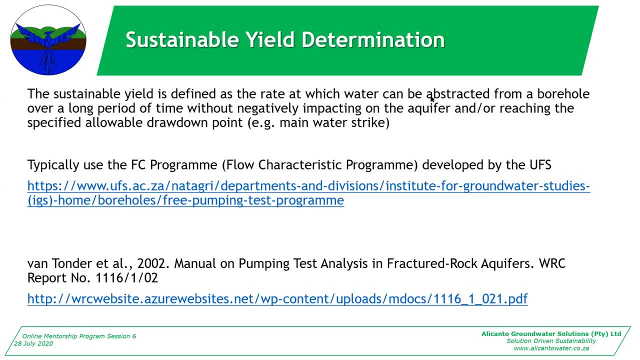 For example, your main water strike. Does that definition make sense to everybody? Yes, Yeah, it does, Looks like it does. Yeah, it looks like it does. So it would be interesting if you could explain what that would do. So it'll just take the water. you know it's water removed all of a sudden off the surface of the surface of the surface. 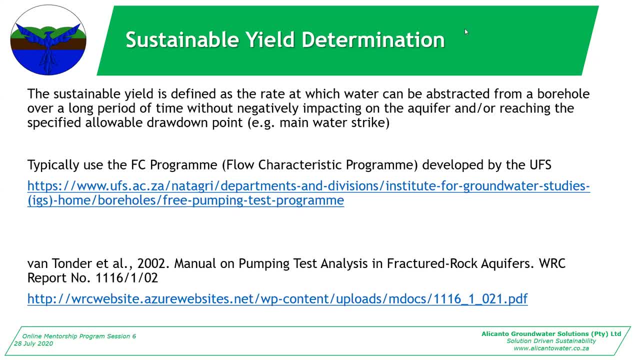 So you're looking at whether you're going to have a water return or not, And you can use a water drain. You can use a water drain to work on that. Yeah, so that's how it works out for you. yes, it does. yes, yes, okay, so you can't take more than there is. 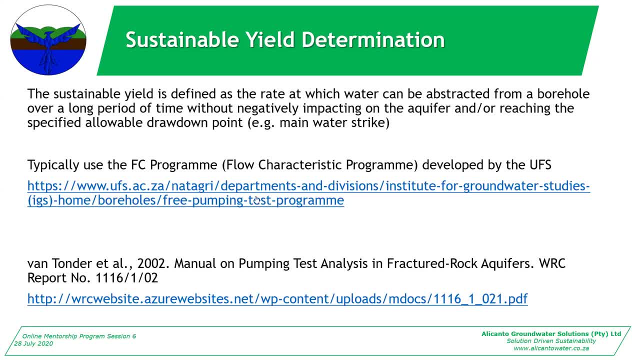 okay, we typically use fc. like i said, this is the website link for the program. it'll download a zip file with the excel spreadsheet. and then here is the manual on pumping test analysis, the wrc report by fantonda et al from 2002. this is a direct link to that, otherwise you can just. 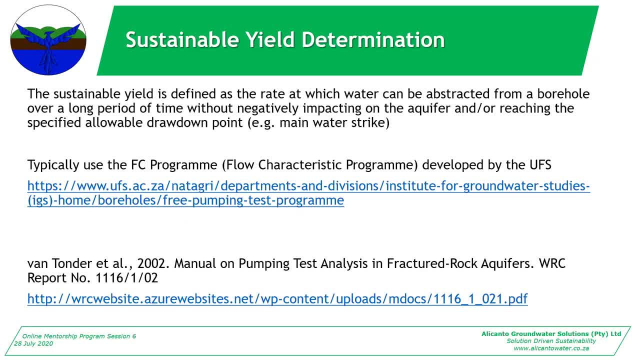 go on the wrc website and search in the knowledge hub, you'll get to this. it's a useful manual and if you couple this with your chris and one and the ridder that we spoke about in the previous sessions, that's definitely definitely worthwhile. the question here: calculate the drawdown radius from antonio? antonio, i'll get to that. 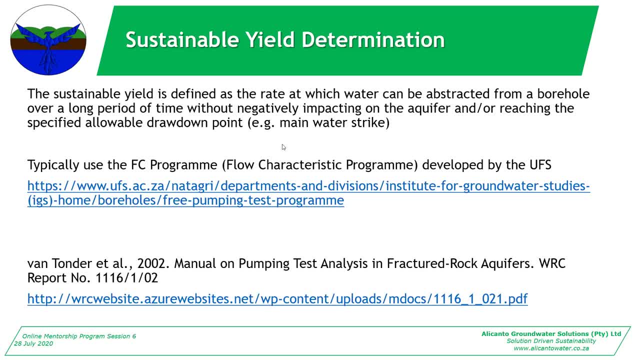 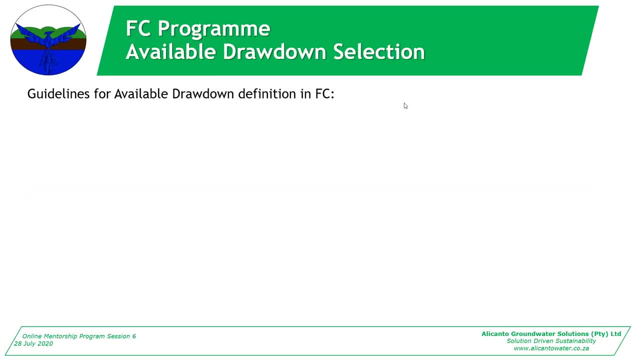 just now because that's related to your cooper jacob, so i'll just show you that in the cooper jacob. okay, so the guidelines to choosing your available drawdown: yeah, we mentioned in the previous slide that your available drawdown is important for your sustainable yield. 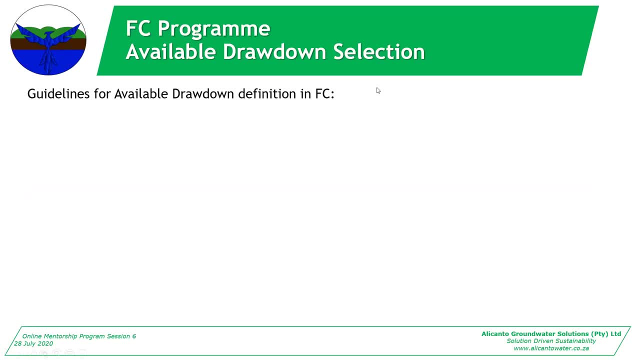 the way you choose your available drawdown. does anybody have any suggestions? how do we determine the available drawdown? uh okay, there's uh sort of like many methods that you can use, and there's this, there's a one that you have to use, sort of like a geometric mean, when you don't have an idea of where is the water's. 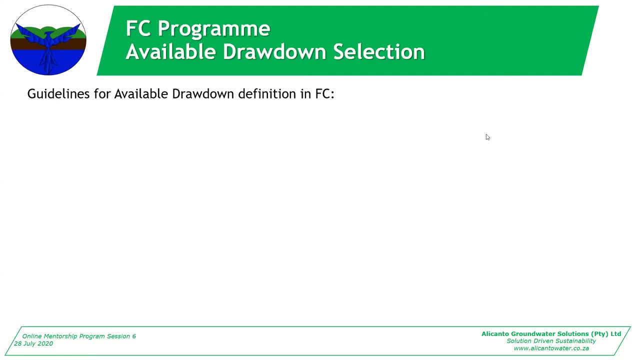 right. so sort of like. you just have to calculate a bit about geometric mean when you have your static water level and the depth of the pumping, something like that. there we go, so geometric mean between your maximum possible drawdown, which is your pump setting, and then your static water level. 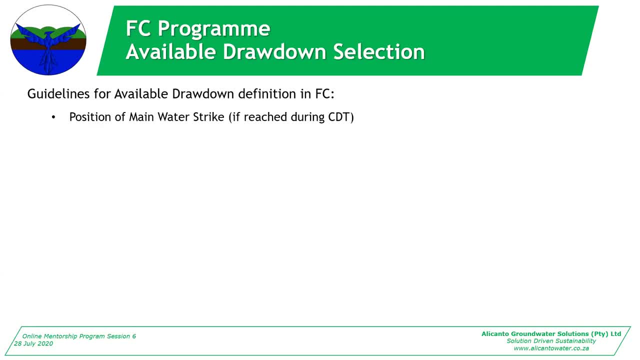 okay, the position of the main water strike if you've used, if you reached it during the constant discharge test. yeah, antonio says the point of inflection on the graph, the drawdown graph, which is correct, where you get a sharp increase, so where you start de-watering your borehole. 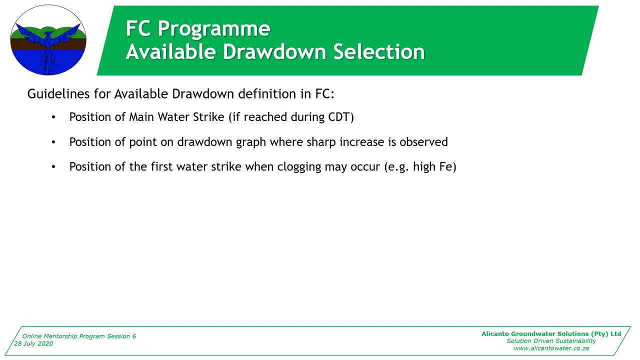 then, in the the event of a possibility of clogging, you're going to do it to the position of your first water strike, that's, where you've got high iron content, high biofouling potential, something like that, in your groundwater. then, if you're borehole recovery flats, 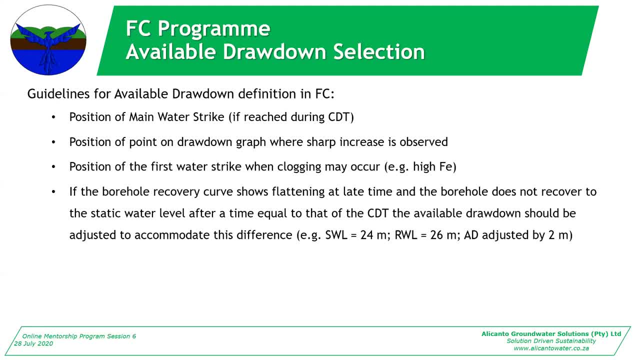 flattens in late time in your recovery test and the ball doesn't recover to the static water level after a time equal to that of the constant discharge test, the available drawdown should be adjusted to accommodate this difference. so, for example, if your static water level is 24 and your borehole recovers to 26 meters, 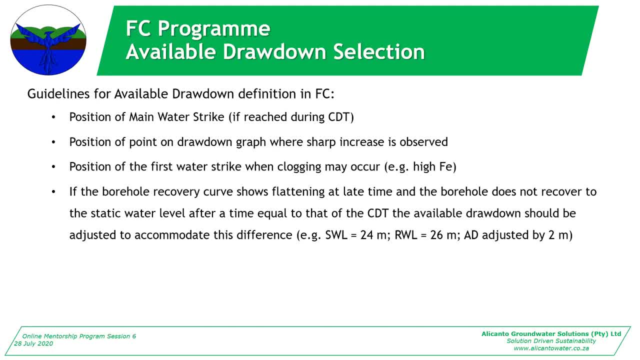 then you need to minus. whatever you calculate your available drawdown, you need to minus two. does that make sense to everybody? um, yes, matthew, it does, awesome, okay, and then in dolomitic aquifers, rule of thumb, you take five meters as your available drawdown. 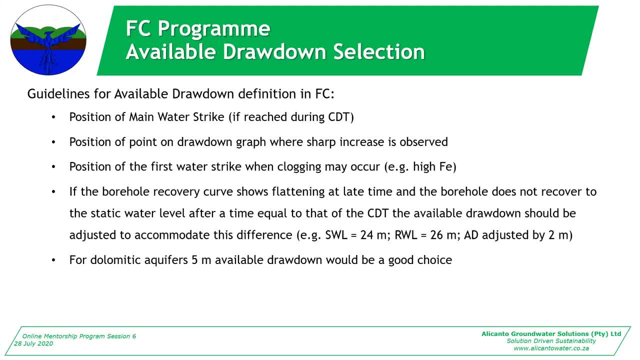 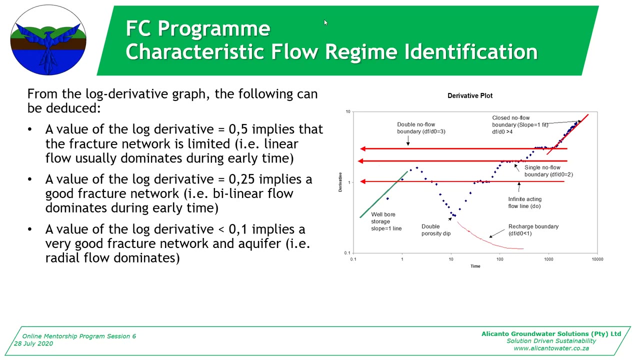 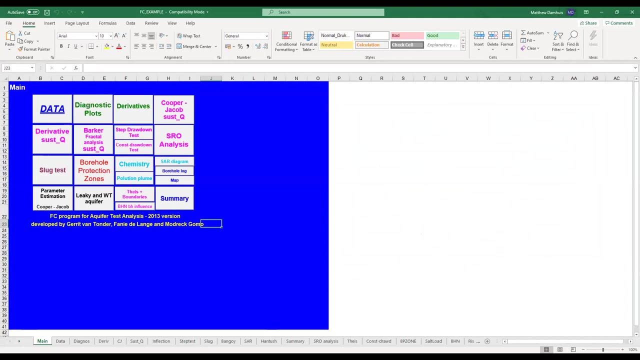 that's just to prevent sinkholes forming. yeah, this is um, just sort of a rule of thumb. according to fontana in the 2002 paper, that's where you've got your thousand plus transmissivities and that kind of thing. okay, let me show you the um fc program. okay, can everybody see my excel sheet now? 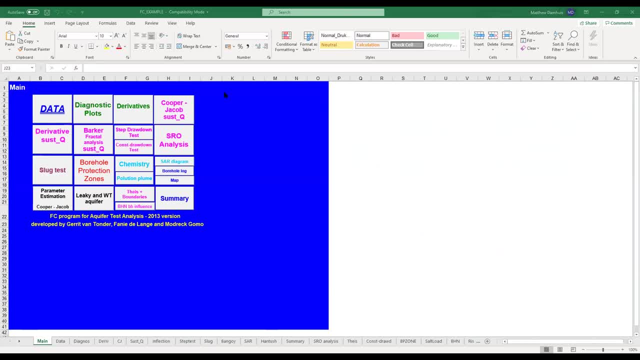 yes, sir. okay, great. so this is the main menu of the fc program that you can download on that link. so you can see i've got data, diagnostics, plots, diagnostic plots, derivatives, cooper, jacob, sustainable yield derivatives. sustainable yield, barker analysis, step test, slide test. you've got a slide test. 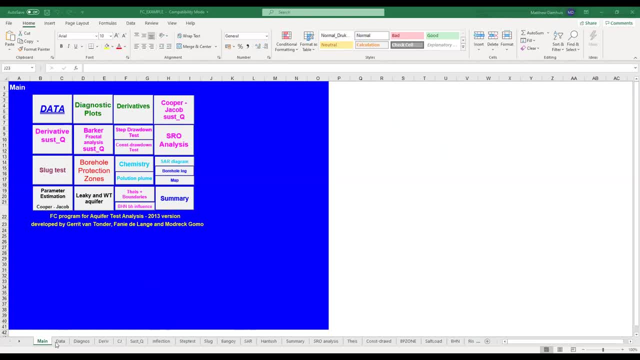 interpretation there and then the summary. so the ones we typically use is your data. this is the example that we are using in a cross being, which is our protocol, and you can also use data for compartments. this is your stimulation for that. and then, in case we add it to the Rain folic fluid. identify the technique. you want to have the65 certified exam engineer separately appropriate Cyça supplies. follow the your data categories. we would want to have the efficacy press up here which shown in the gaativa um alpha and beta. monetary Heckler have found is this: it's so: built man two drill block and I would like to highlight the frequency baby, but on average that up to a 스� applause have a single covid. these kind of heh we're now, Но that's it. 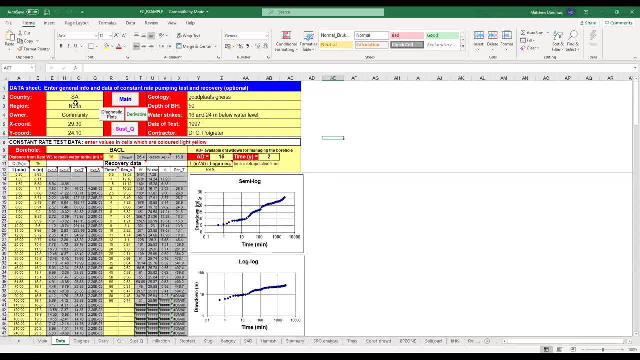 you download. so you fill in all of your borehole data here: borehole name and then this one. you physically fill in and you can see here it's calculated. your recommended available drawdown is 16 and then you fill in here based on the recommendation. you know sometimes you'll put in a 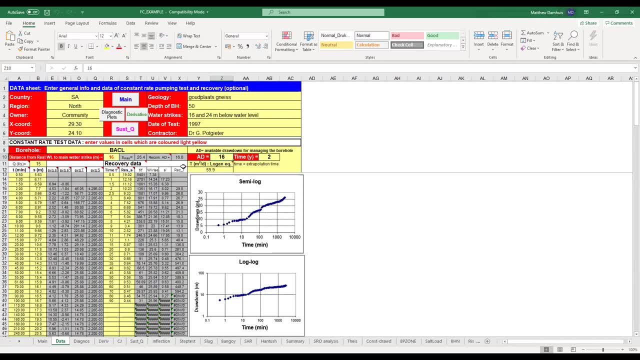 water strike distance of 24, but it'll still recommend 10.. so then you can choose. do i want to take mine or do i trust the program? then your extrapolation time: your minimum two years, but you can set it as 20 years, 10 years, depending on the life of your project. if you've got a farm, that's. 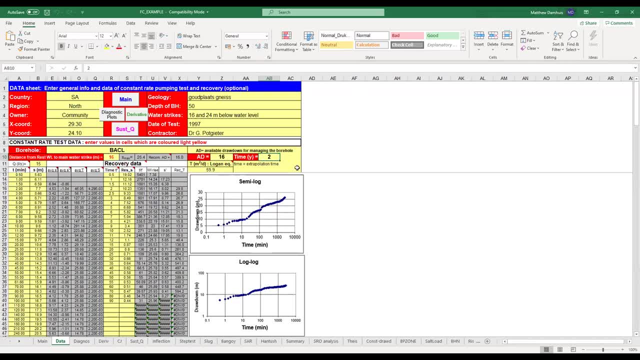 going to be productive for 20 years, then set this extrapolation time as 20 years because, remember, the definition of sustainable yield is where it can sustain this yield over time. so the longer the time, the more conservative you're being then. this is your abstraction rate during the pump test over here, your drawdown data: 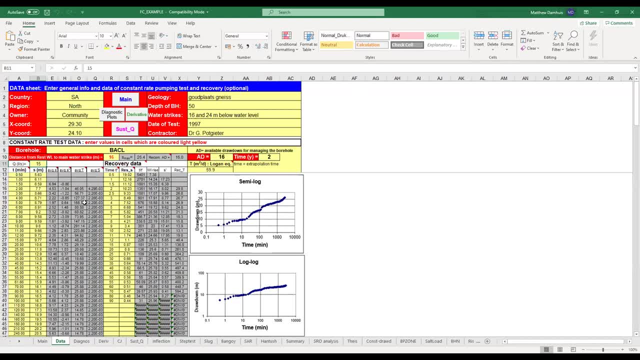 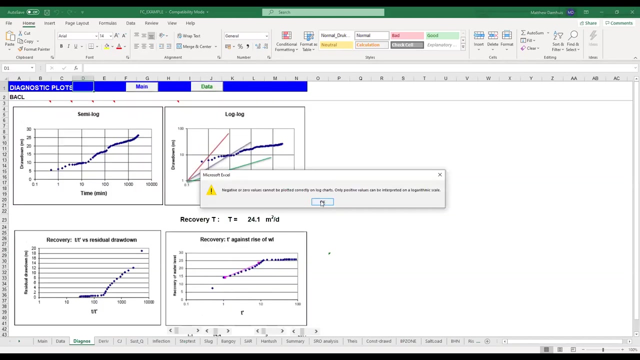 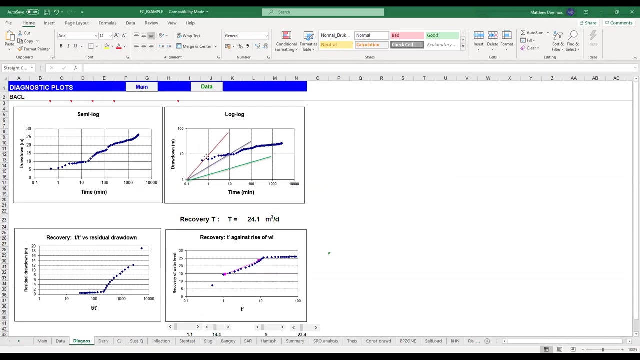 and your recovery data. leave these gray cells alone. these are the calculation cells. everybody comfortable with the data entry in fc? yeah, thanks, cool. okay, then you can go to your diagnostic plots. i don't know why it keeps telling me that, but then you've got your one to one line here to measure your one to one gradients. 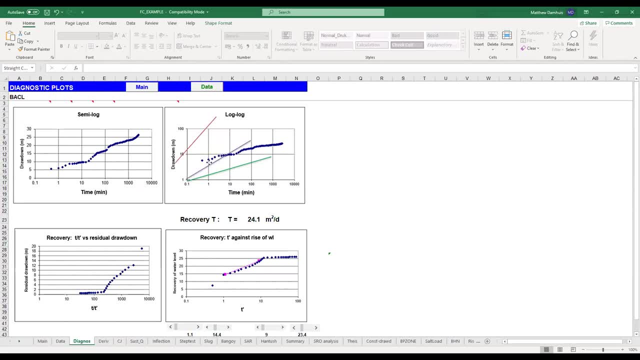 and you've got your one. what's this one about? one to four here. so your 0.25 gradient and this is your 0.1 gradient. so that's the first derivative graph that you can see. so you can see on the graph if you go to your data in your data center. 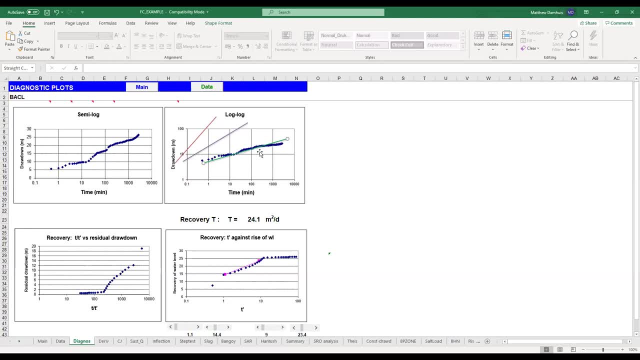 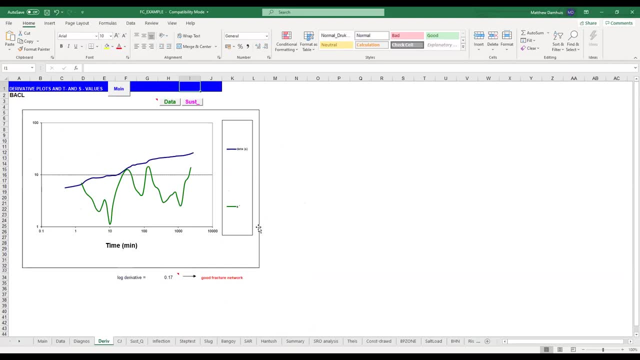 so that's the first derivative graph that you can see and you see here that fits on that curve. okay, we'll go back to powerpoint just to explain. well, let me show you the derivative graphs again quickly. so here is my data on a log log diagram. so there's my raw data. 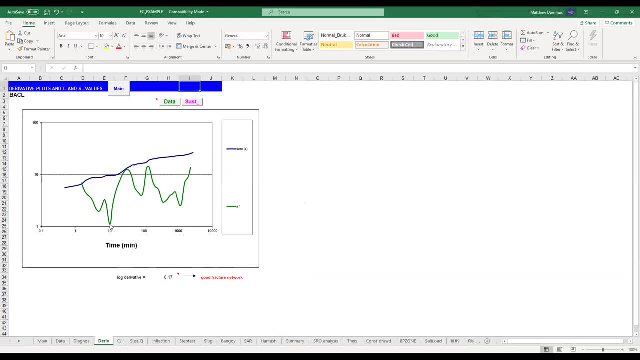 then here's my first derivative data: fracture being dewatered, fracture dewatered, fracture dewatered, fractures dewatered. You see, there it says log derivative is a good fracture network. So just remember this, because I'm going to go back to the S-Clingy way. Matthew can. 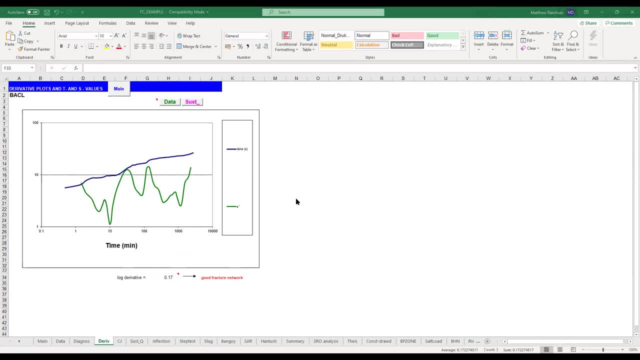 I can you just please explain why the derivative, why that the low point means mean that the fracture is dewatered. I'm going to get to that. I'm going to go back to PowerPoint just to explain that, But I just wanted to show you where it. 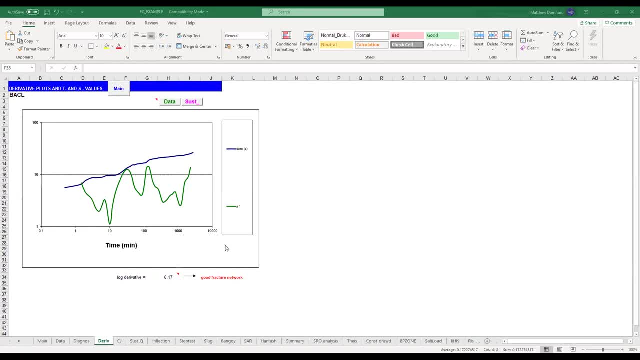 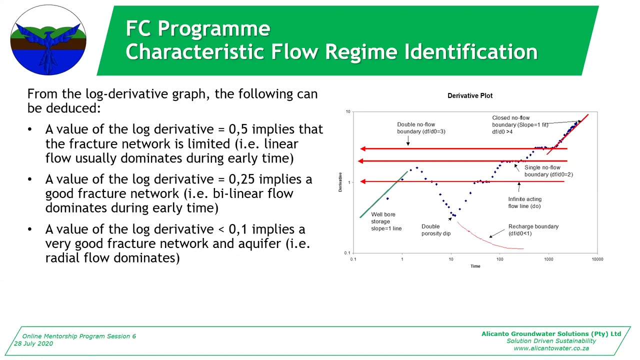 is in the spreadsheet and then also what it looks like. Okay, Sorry, No stress, It's a, it's a question that I'd ask as well. Okay, Everybody see PowerPoint again. Yes, Yes, Okay. So from the log: derivative graph. 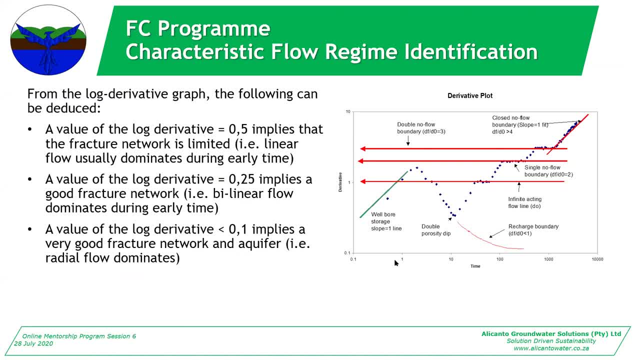 which is that one that I just showed you. there you see log of derivative, log of time, And here's my first derivative graph. here, Value of log derivative 0.5 is a fracture, network is limited and it's a linear flow. 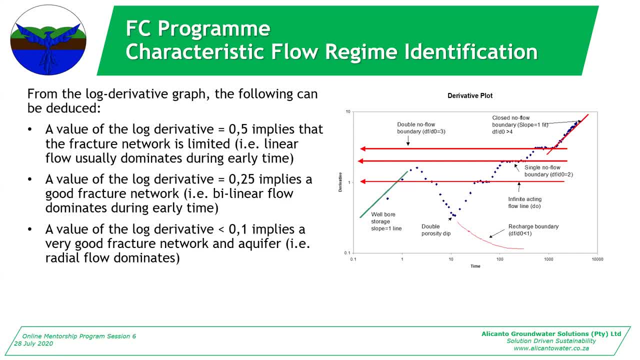 So where you've got a gradient of 0.5, then you've got a limited fracture network log derivative of quarter. So one to four implies a good fracture network. So bilinear flow, that's the one that remember I showed you. Ah, those different colored graphs in Fc, or lines on the graph in FC, That's your point: 5.25 and 0.1.. 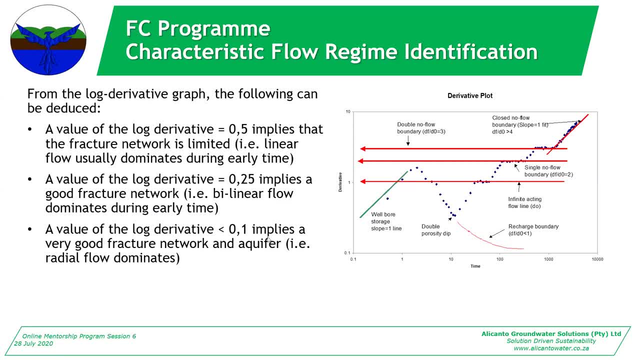 so we've got log derivative of 0.1 or less. that's a very good fracture network and the aquifer. so you got radial flow. so flow is coming in from all sides. here we go. slope of one in early time is your well bore storage. you've got this here. 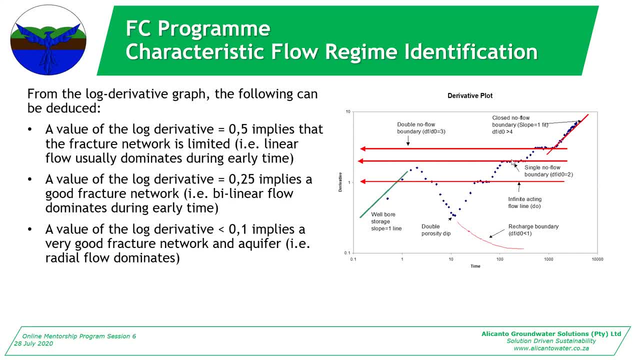 double no flow boundary, single no flow boundary. you see how it flattens out here in your closed no flow boundary is where you get a slope of 1 in late time, so that's where you do watering it. you think about what's happening in the bohol. your water level is dropping, your drawdown is increasing, so you're gonna. 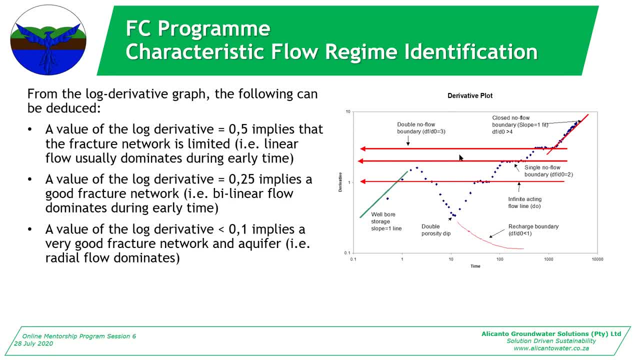 get this straight line and that shows you a closed, no flow boundary. you got your dual porosity dip. so that's why I'm saying your fractures are D warts it you're Jill. you've got matrix flow and fracture flow, so you get a dip where the drawdown decreases over time. 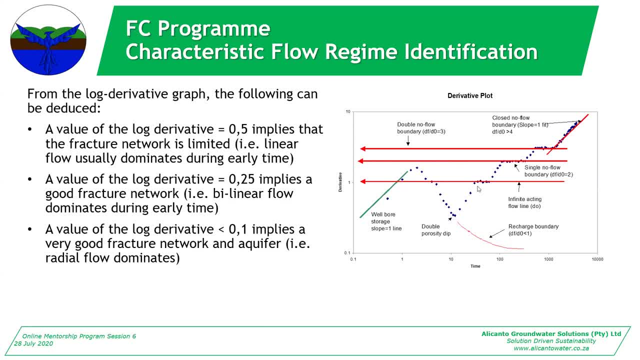 and then it increases again. so you dewater your fracture there. then you start getting drawdown again. does that make sense? um, i'll think about it. i'll think about it, like you can continue and think about what the graph is showing. it's showing your derivative of your drawdown on the 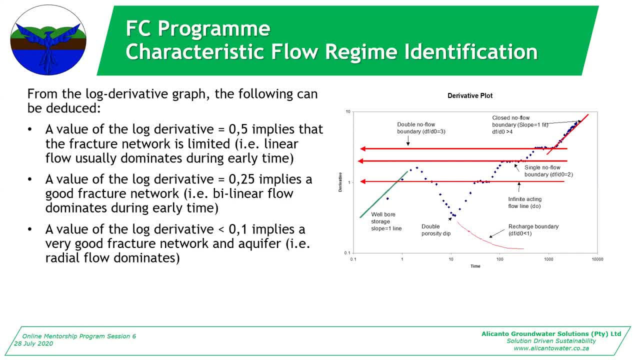 y-axis, so your drawdown will increase when it's dewatering. so water is going out faster than it can come in, then it'll stabilize. when you get a fracture or a water strike where you're starting to get equal to your pumping, then you dewater that and it'll increase again. so just think about. 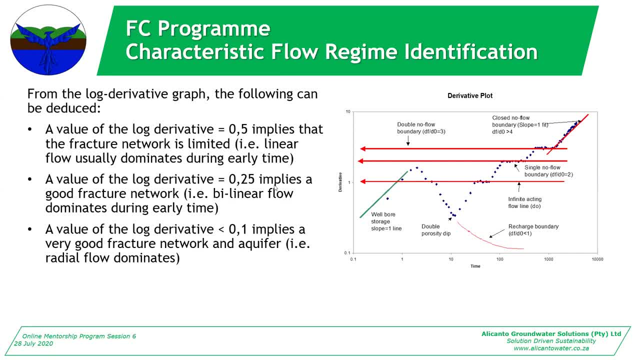 what's actually happening in the ball hole while you're pumping it. so you have it. read the read like: but read that font on the paper. that summarizes it very well. let me just check. okay, so then i'm going to go back to excel now. just show you, we'll go through this fc example together. 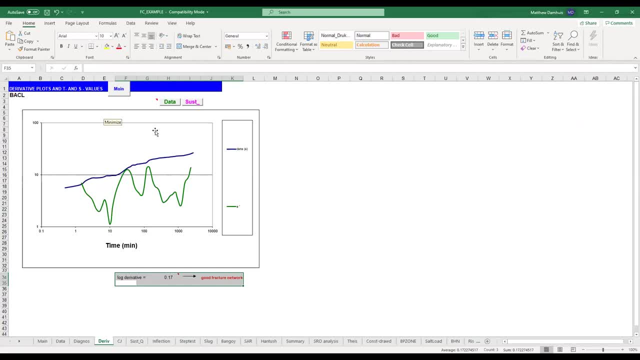 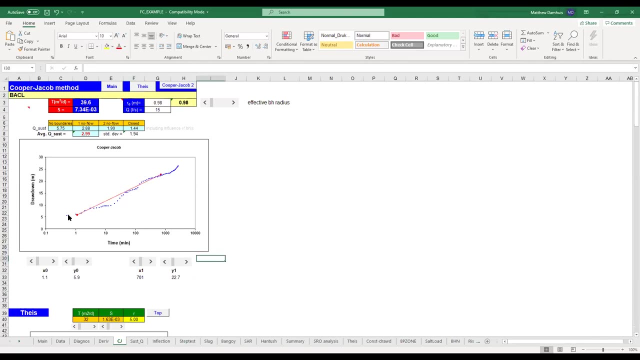 okay, everybody see excel again. yes, cool, okay. so here it tells me i've got a very good fracture network. now we're going to go to this cooper jacob method where you fit your line graph here. now the way it fits in the newer excel is quite cumbersome. you see, here's my wire. 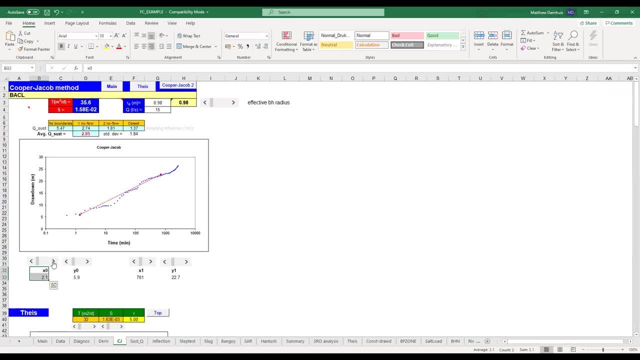 and my x for 0.1. so you'll see if i move that it moves around, and then the y as well, you can see that moves around. so it is quite cumbersome. but try to fit your line as best as possible because otherwise you can just type it in. but the trick is to type it into this k7. if you type it in. 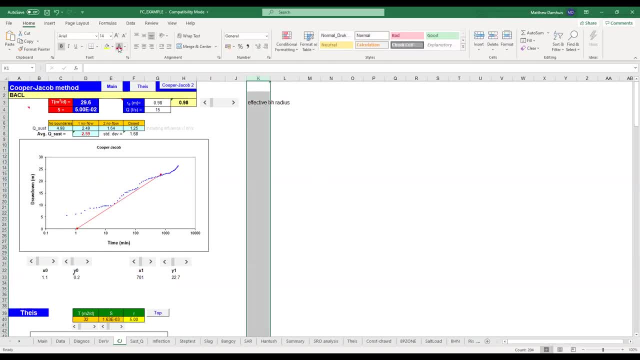 here. it doesn't do anything, okay. so there's my x zero, 0. there's my y, that's my x 1, then y zero. so you can type it in manually if you want to here. that's just to fit your line. so i'm going to put it back on 5.7. 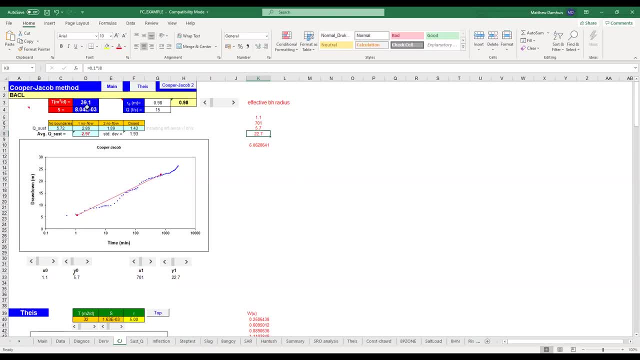 yeah, so then it fits good. so here's the gray kind of flower. there you can airplane kind of flat break to the left, to right, to right, to right, to the left, to the left, to right, to the right, to right, to the right, to the right, to the wrong, to the wrong. creating an arm job is very easy, but of course you can fit that back specifically. so R as and over here it's in on the name of the delayed step. so we're just going to go ahead and cable the table to go away and you've got our. 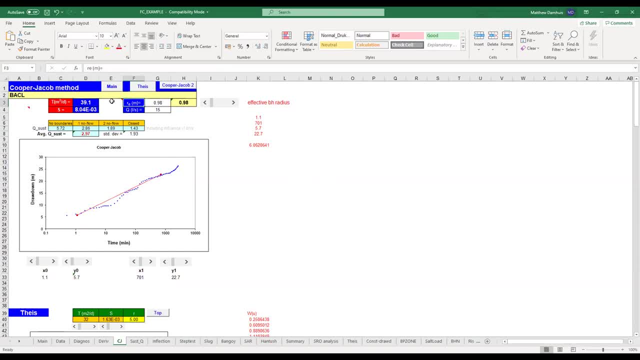 then it calculates my transmissivity and my sustainable yield with no boundaries. one no flow to no flow or completely closed gives me an average sustainable yield of two point nine seven liters per second. so that's the Cooper Jacob method. you just fit your line like you would if you were to interpreting for. 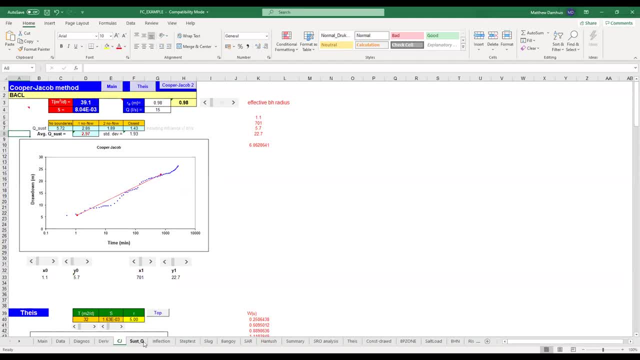 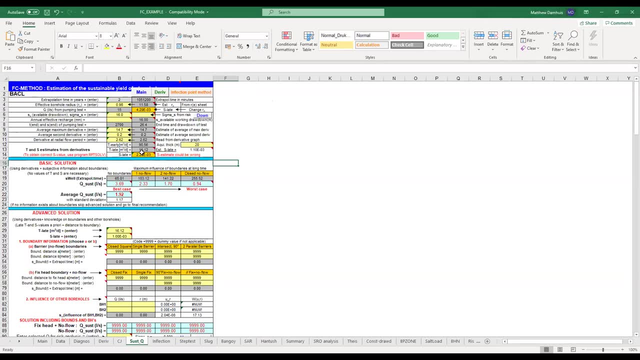 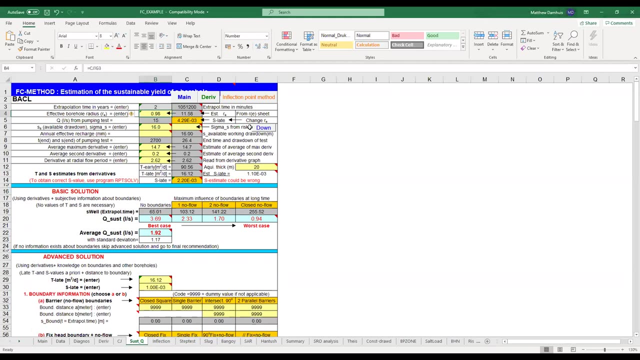 transmissivity. and then here is the FC method. you know this is the sort of unique method that the Free State University developed. so you've got your estimated effective borehole radius. this is your extrapolation time from the data sheet. so two years, if you type in 20, that'll. 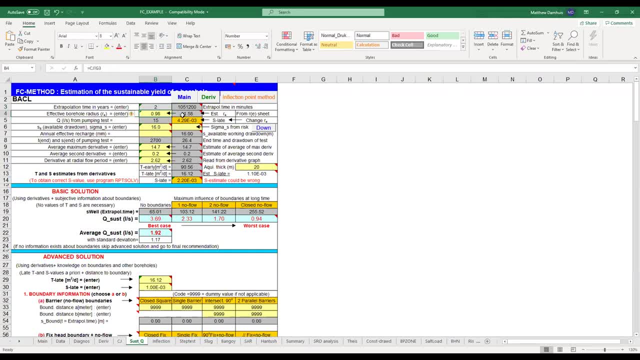 change to three years. if you type in 20, that'll change to three years. if you type in 20, that'll change to three years. if you type in 20, that'll change to 20 effective borehole radius. you can calculate it on this re sheet. but 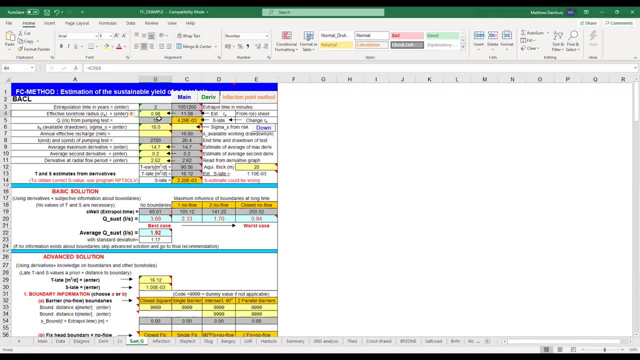 typically you just leave it as the default. then your cue, your pumping test cue, which is what you've put in at the data sheet, same as available drawdown on your data sheet and your effective recharge, that is, if you know what the recharge rate is at the site. 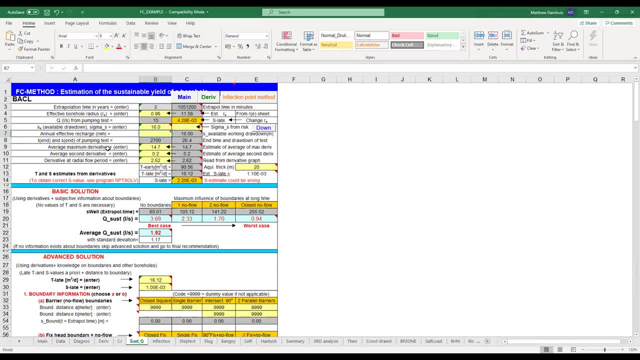 you know you've got 20 millimeters per annum. you can put in 20. you see, the units here are 20, but to be truly conservative, you want to leave that as zero. yeah, does anybody have an issue or a question about why you leave recharge? 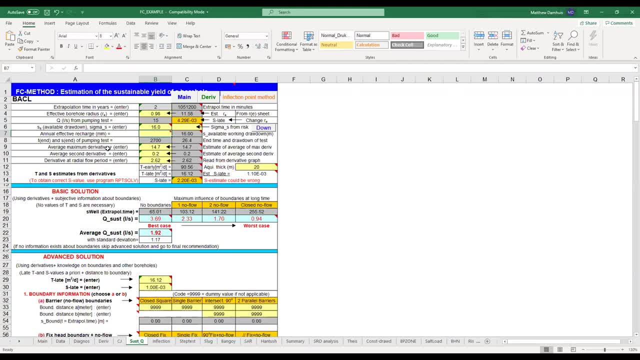 is zero chances. no, okay, so watch what happens if I put no okay, so watch what happens if I put recharge in. you see, my average is 1.92 now. so if I put 15 millimeters it almost doubles. you look at that. if I've just got 15 millimeters recharge per annum. 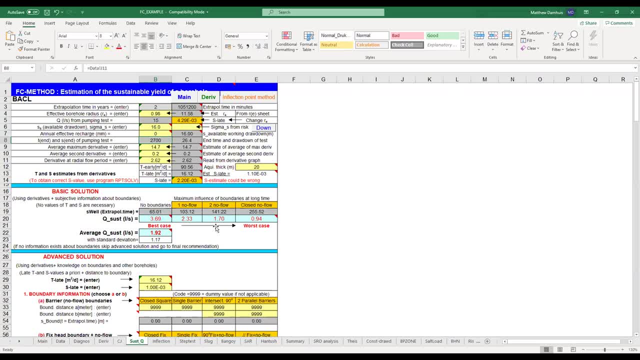 knowledge. suppose you have an average of 1.92. you see my average. you see my average is: yeah, i mean, look at that. so to be conservative, leave it as zero maximum derivative. it calculates off of the derivative trots second derivative as well. these ones you just leave as default unless you really want to. 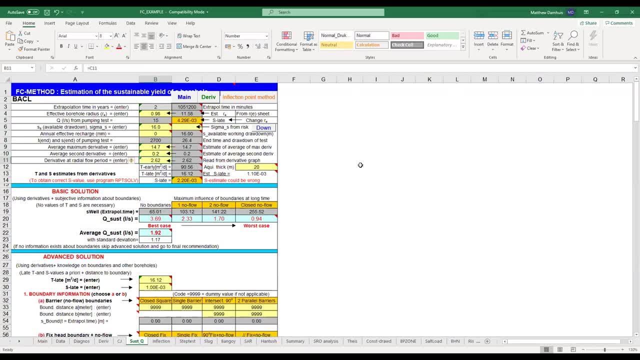 go into the maths, yeah, which i don't usually do. then your aquifer thickness, you decide based on your drilling log, your borehole log. is it a fracture where it's like five meters thick zone, or is it 20, 30 meters? you decide that based on your drilling log and then it estimates your. 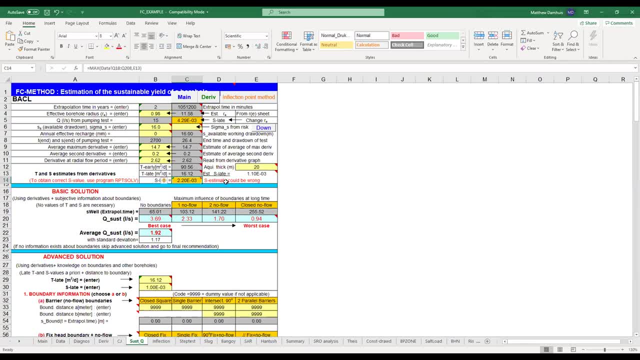 storage. and it even says: yeah, the estimate can be wrong. so that's where you need an observation borehole during your pump testing, or you can use rpt. solve you. that's the recommendation of fc, but i personally just leave it as default estimate. okay, then here's your basic solution again. 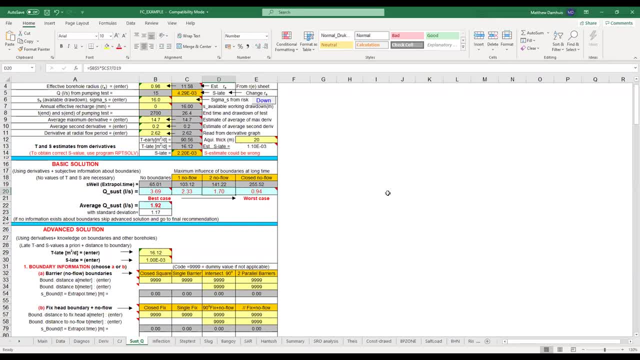 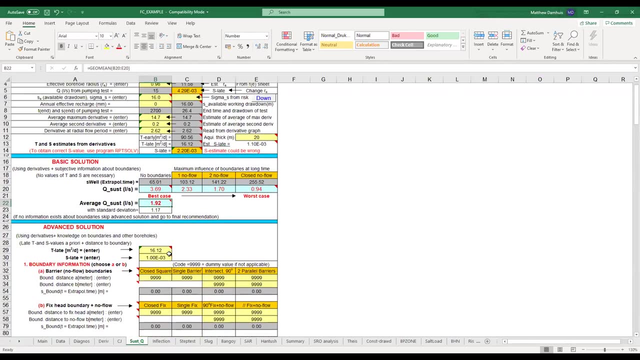 no boundaries, then your one no flow boundary, two no flow boundaries, then a closed no flow boundary and it gives you your average here. i'm not going to go through the advanced solution because personally i've never used it. yeah, usually the basic solution is good enough and you don't have enough data really to do advanced solutions. 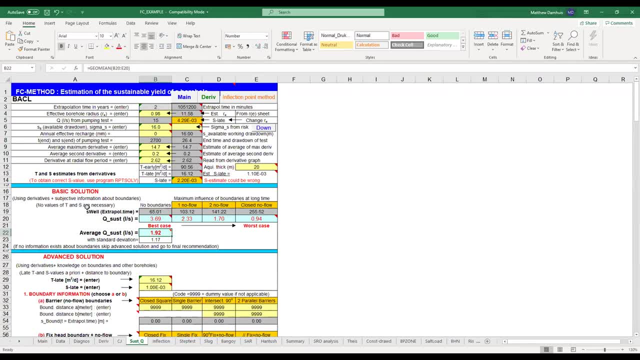 everybody sort of okay with the data that you put into this fc method, the basic method, yep, yep, okay, yes, yeah, great, look, it's pretty straightforward. so i'm not going to go into the maths and that stuff because that just confuses everybody, including me. 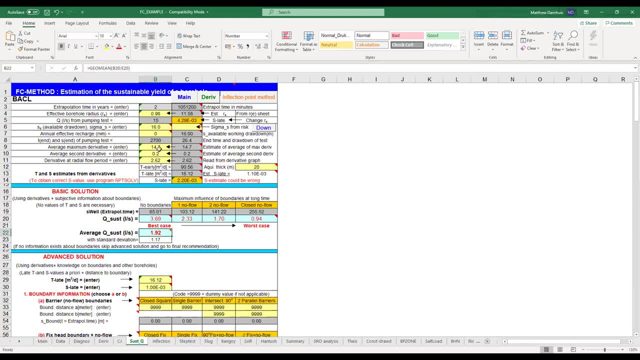 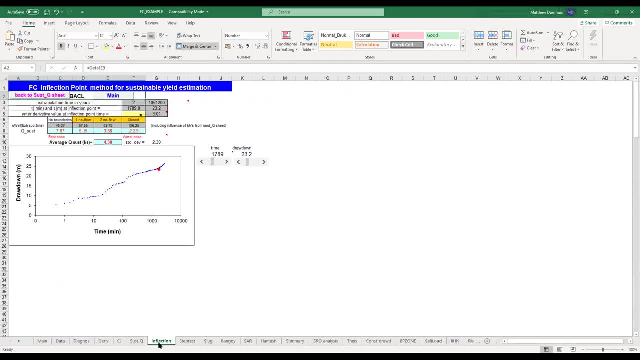 so this is the way they've built it and it's been accepted, so i'd rather just focus on teaching you how to use the software. the other one that we use is the inflection test, which is what we mentioned in about determining your available drawdown. 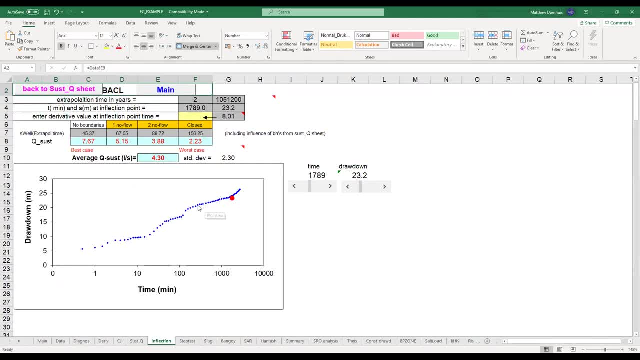 you can see here inflection point. you can see it's on a log time and a linear drawdown so it goes and then it starts increasing. it looks a bit, just goes up, similar to here where you've dewatered your fractures. as you see it's stabilizing. 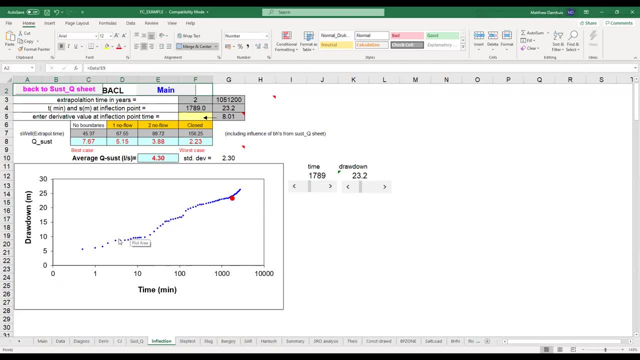 can give you. this is what I was saying on the derivative graph. you've got a fracture that's yielding a decent amount of water. you need the water that fractures. so you drop down your water level. then the fracture starts to almost meet your sustainably or your pumping yield. the dewater that fracture. then 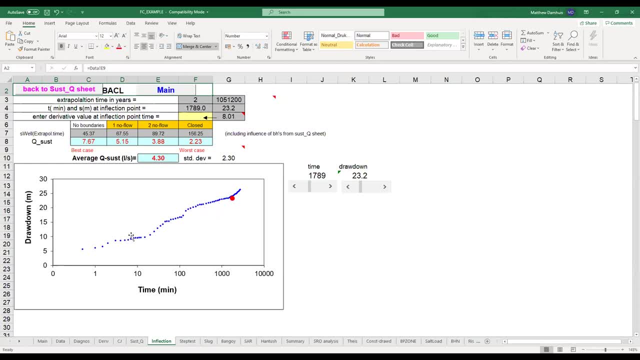 here you've got another fracture that's a bit higher yielding than these ones because it lasts longer. then, yeah, you've dewatered that fracture and you're going down towards your main water strike or your pump in it. now I see it great. always take a step back from the, the data and think about. 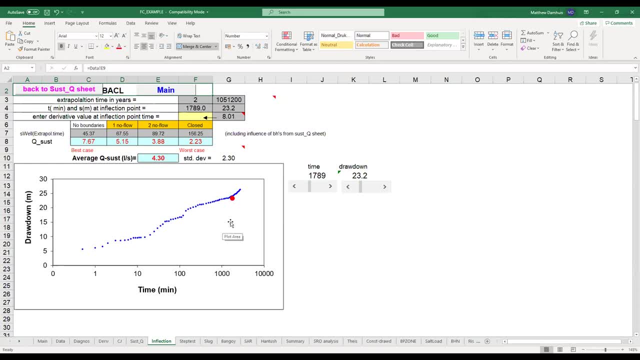 physically, what is it? it's a borehole with water going in from the geology and being pumped out by the pump. and then think about it in those terms. forget about the maths and the graphs for a second and just physically think about what it is. yeah, they don't know. thank you, I see it actually. yeah, I know once. 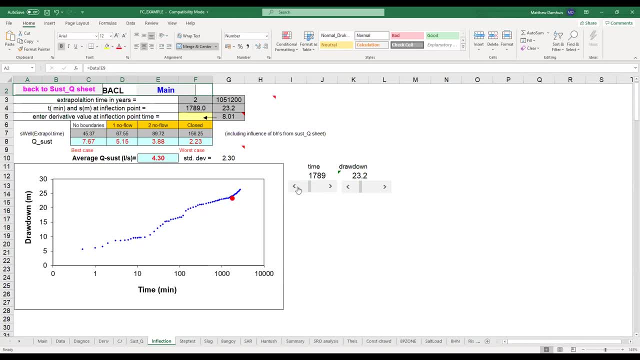 you see it and you think about it in the terms that suit you best. then it makes sense. everybody, like I, like the maths, but some people like the physical side, some people don't like the physical side, some people don't like the physical side, some people like the graph side. that's just finding your. what talks to you? you. 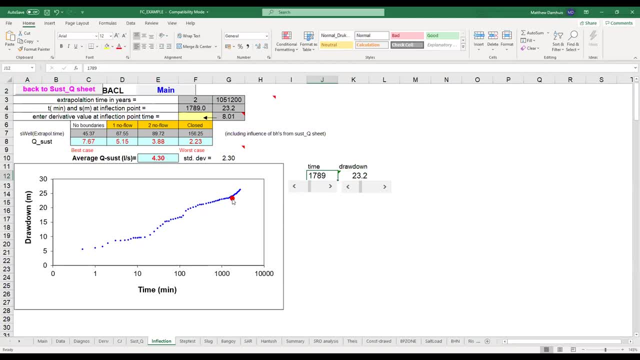 know okay. so again, yes, you move the dots around with this. it's not making a big difference here because you in the thousand to the ten thousand on the log cycle, so you can drop it all the way down there. see you, look at our changes, my results as I go along. 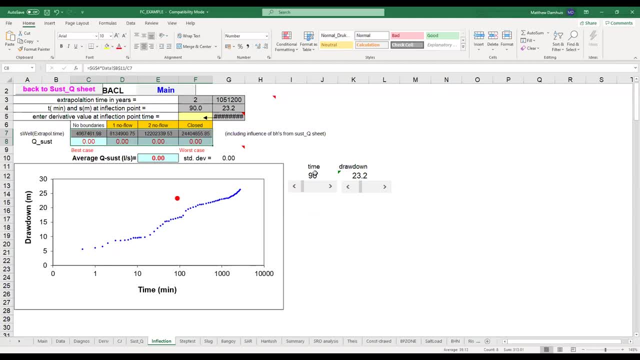 put it back on. does it 1785? yeah, there we go. but you see, here again it's a lot higher than the other estimates. so I don't like this one because they you might have another fracture hanging around. yeah, you know, this might be completely dewatered and this doesn't recover, so I personally don't like this. 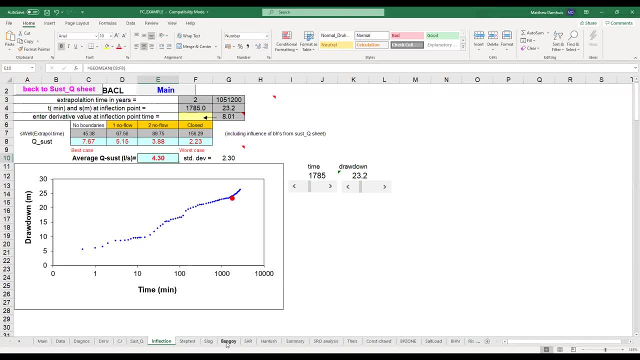 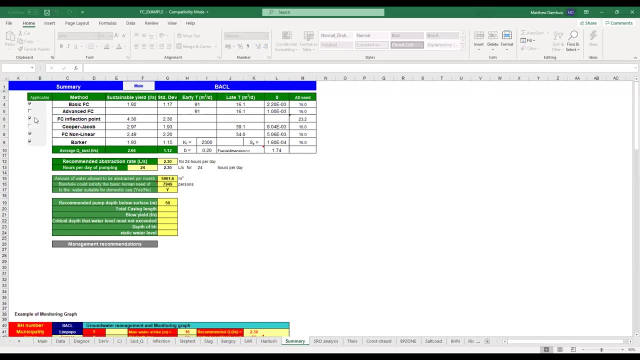 inflection method. I'm gonna ignore those. then we're gonna go to the summary. you see, yeah, it's got the check boxes for the basic FC method. that's the average yield, that it's calculated. inflection point: that's the average Cooper Jacob, I want that one if 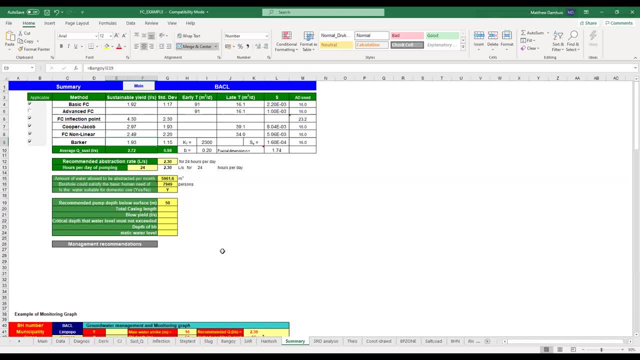 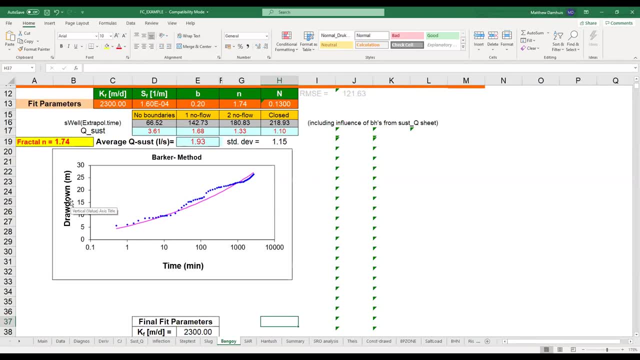 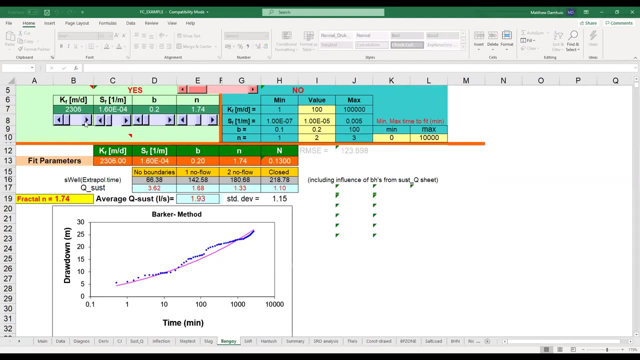 seen on linear and then the Barker method, you know. so that Parker method is here. I don't use this one that often, but the way you can adjust it as well. you see, there's my K that flattens my curve. the higher it goes, the flatter my curve gets. 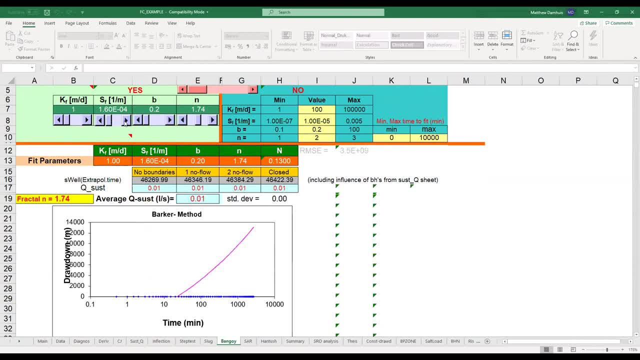 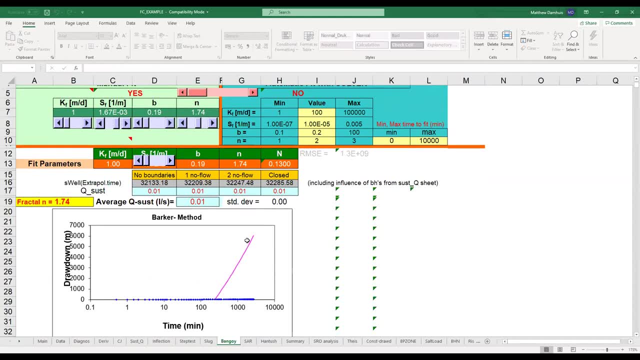 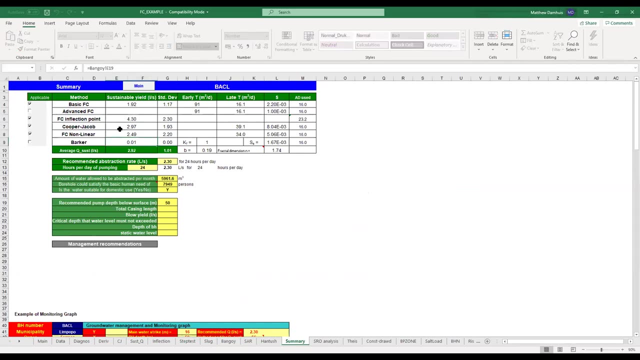 and then your storage, your thickness here and then your in again. I don't use this one but you can for the look with it, if you want to use it, if you want to use it, if you want it. so I'm taking the average as FC nonlinear, the inflection. 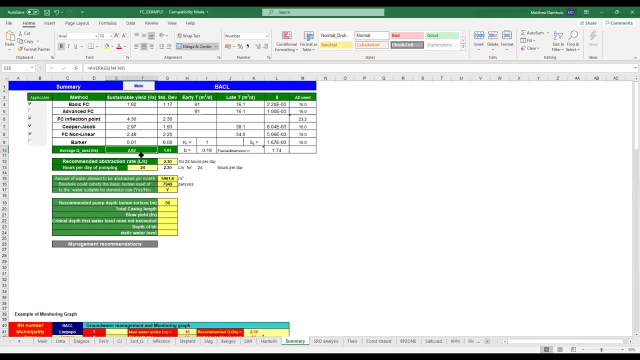 point Cooper, Jacob and basic FC. so it gives me an average of 2.9. then I just like to type in this one manually. I just say equals that average and that one is for 24 hours a day pumping. so that is flat-out pumping. I mean you're not going. 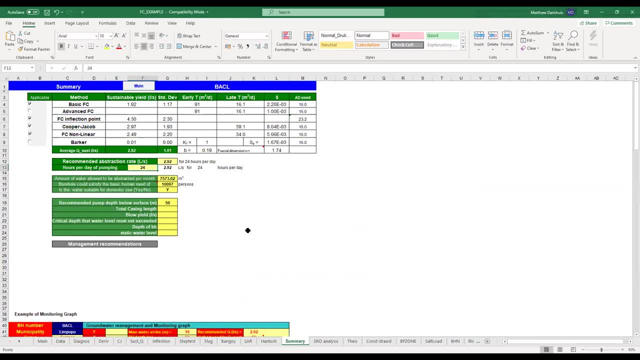 to do that on the site if you you know that's. that's just not practical from a power perspective and a maintenance perspective. so typically you'll do 12 hours of pumping, 12 hours on, 12 hours off. you see how it increases my yield. so for 24 hours it's 2.9 and for 12 hours it's. 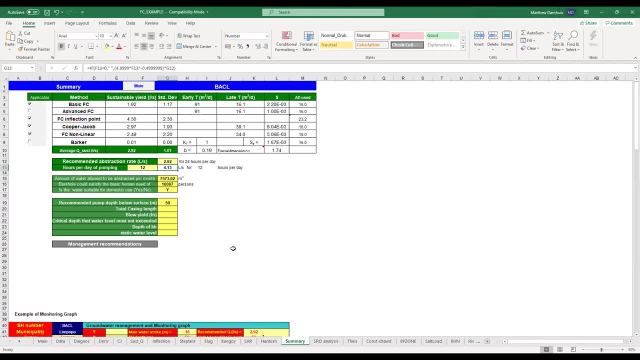 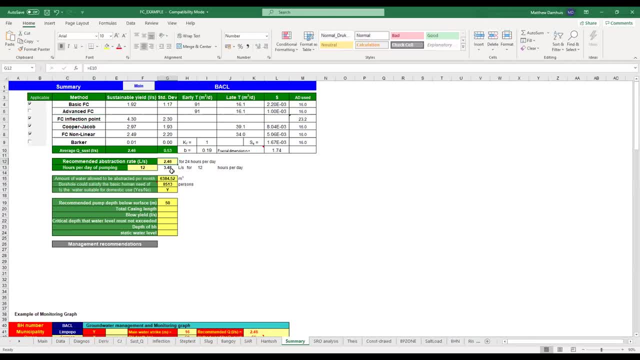 I just turn it off and then it adjust that. but just do this correction, just say equals and then choose this average cell because for some reason in the FC sheet it doesn't do that. and and get a feel for your site, because if you've done your pump test at one liter a second, 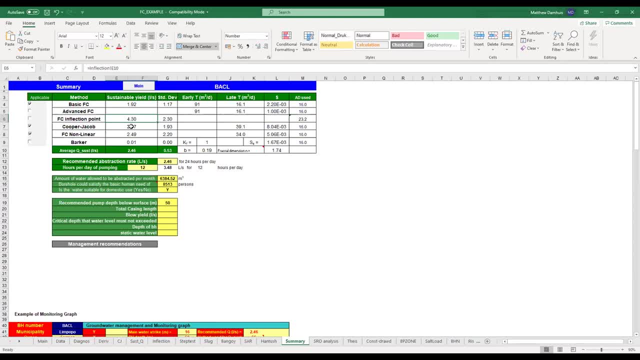 and it's dewatered the ball. your sustainable yield is not going to be three liters a second. you know something has has happened in your data interpretation, so be realistic. your- your sustainable yield is generally not higher than your pumping test yield, unless you're in a caustic system or something. 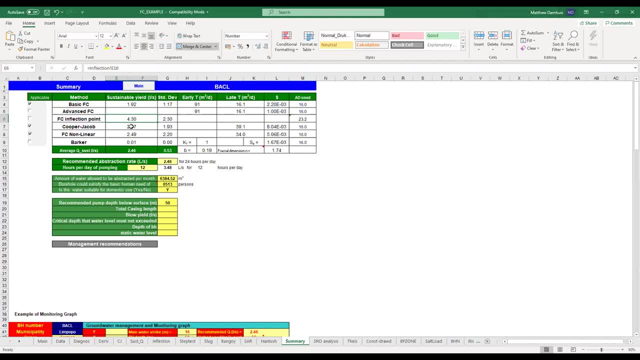 like that. okay, so always go back to your gut feeling. if you don't trust the data, interrogate the data. okay, everybody happy with FC? yes, I'm happy. thank you, Martin. great, any questions about you? know this, because this is just a software package. you still have to fiddle with the data. 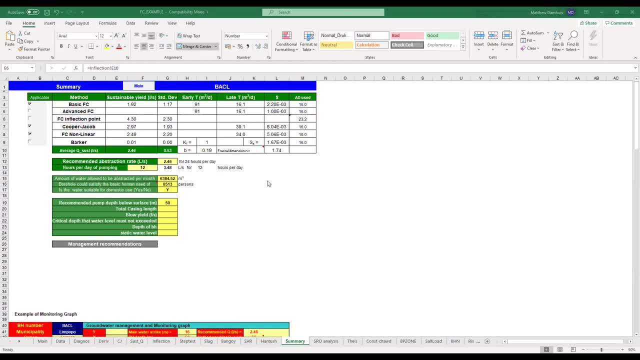 you still need to see if you trust the data or not. I'm just curious to know if are there any other softwares- like specifically in South Africa- that have that are similar to FC or is like FC the like. go to God when you want to do sustainable. 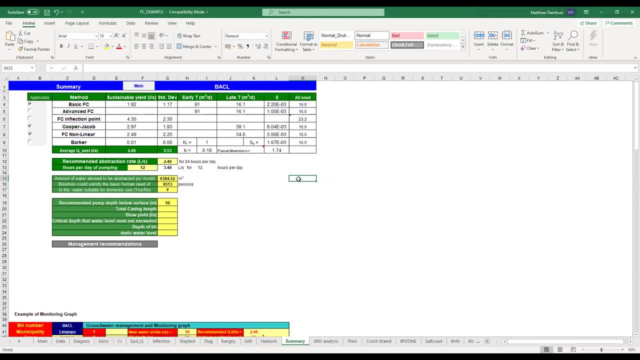 yield. yeah, my personal test data, actually, and my personal experience. you know i was trained in varsity on fc. um, i've used fc on all of my projects. i've used those nf equations that i showed you in the beginning. i've used those as well and they've been fairly successful. 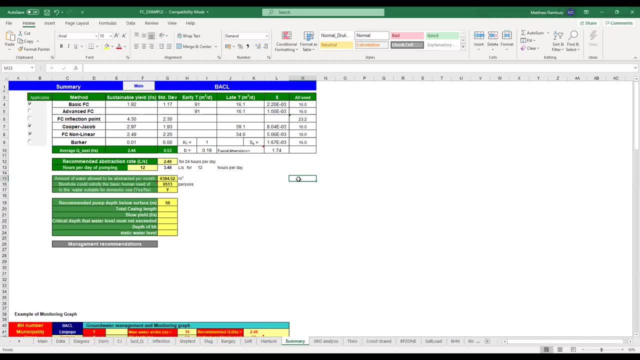 um, you know what i mean by that is that the pumps that we installed, based on those calculations, didn't burn out okay and there wasn't any negative impacts to date- and that was about five years ago, so to date there hasn't been any issues with those equations. 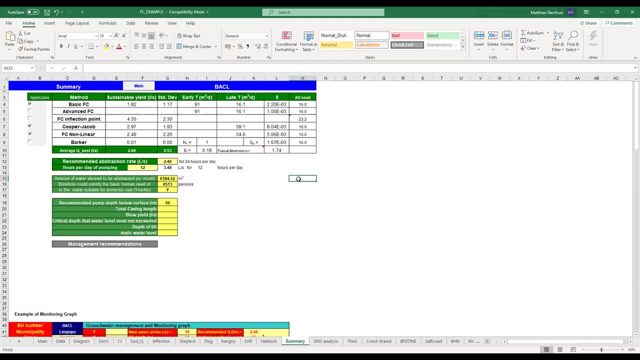 and you know, like we discussed in the aquifer testing presentation, the, the way the farming, the farmer tests, they, they do it, they buy a pump and then they sort of choke the pump and vary the rate until the water level so this stabilizes and that's how they get their sustainable yield. 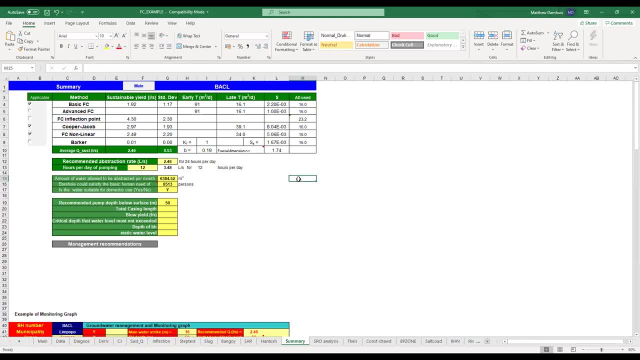 so there are ways. this is a sort of accepted scientific way to do it. okay, thank you. okay, any other questions before we move on? okay, you said something about in caustic environments. i didn't catch that. um, the sustainable yields is usually higher or lower than what your pumping rate. um, you know, for example, if you're in a big 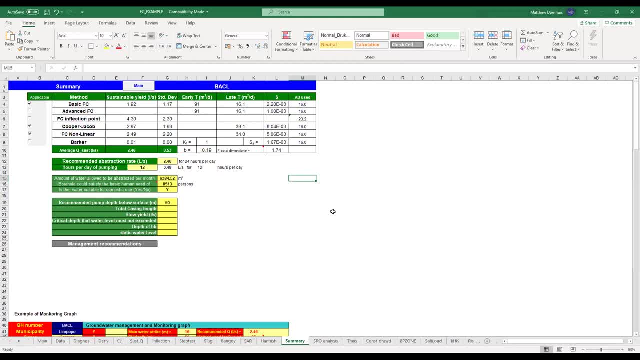 caustic um cavern and you're pumping it like i've had it, where we pumped at 86 liters a second for five days and we had 0.3 meters drawdown which recovered in 30 seconds when we switched the pump off. so the the yield that we could pump that ball at was higher than the pumping rate that we used in. 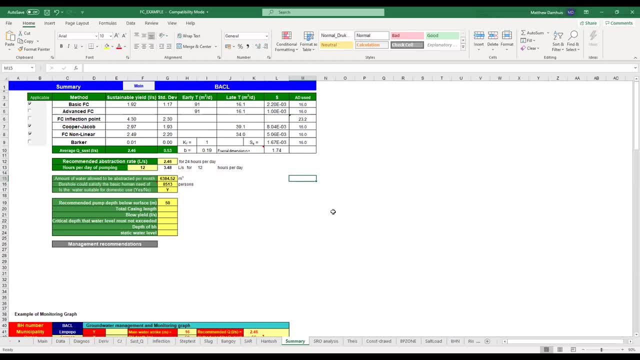 the test. oh, okay, okay, yeah. so in in general, you know we want to. when we do a pumping test, a constant discharge rate test, we want to stress the aquifer. we want to stress it for as long as possible, but we do want to stress it. we want that water level to be dropping down. 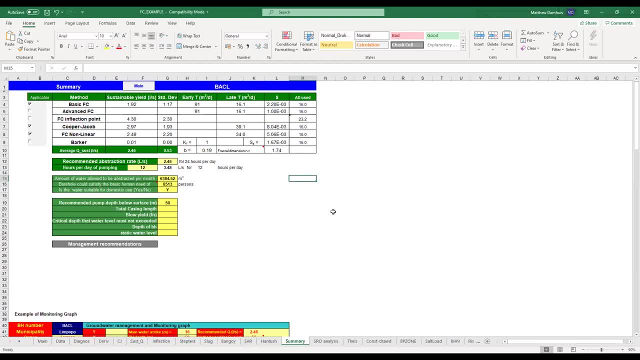 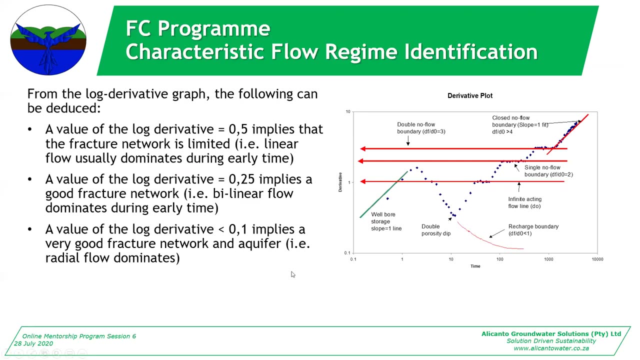 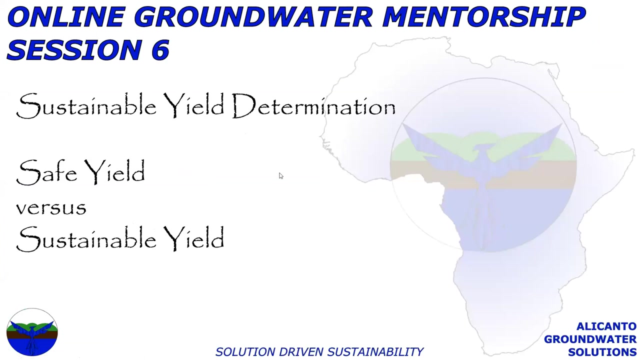 so that we can see its reaction to pumping. yeah, well, okay, thank you, cool, no worries. okay, i'm gonna go back to the powerpoint slide. yeah, everybody see powerpoint again. yes, great, okay, so does. can anybody tell me the difference between a safe yield and the sustainable yield? 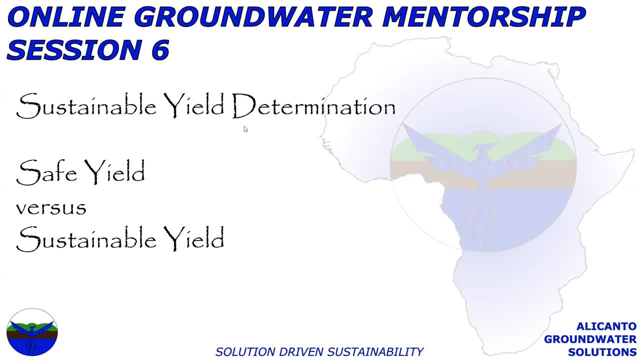 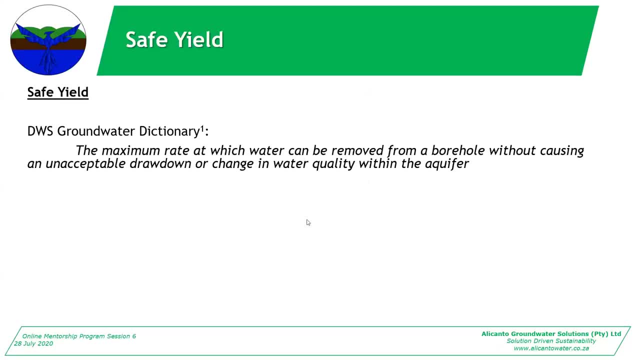 nobody, okay. so your safe yield, according to the groundwater dictionary on the water affairs website, is the maximum rate at which water can be removed from a borehole without causing an unacceptable drawdown or change in water quality within the aquifer and the glossary of statistical terms, the extraction level of a renewable resource which 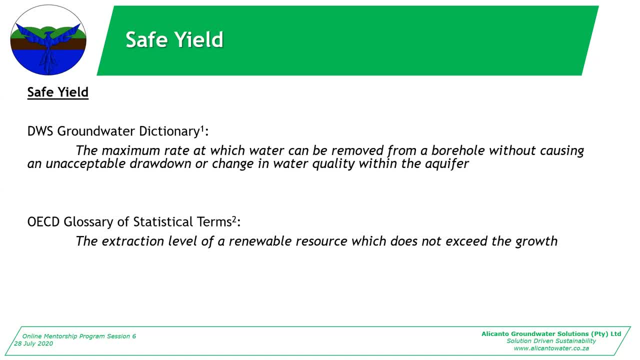 does not exceed the growth. so if you put that in groundwater sort of terms, that is an abstraction rate which doesn't exceed the recharge rate. and here's just a is just a link for those, yeah, on the water affairs website: the safe yield and the sustainable yield. 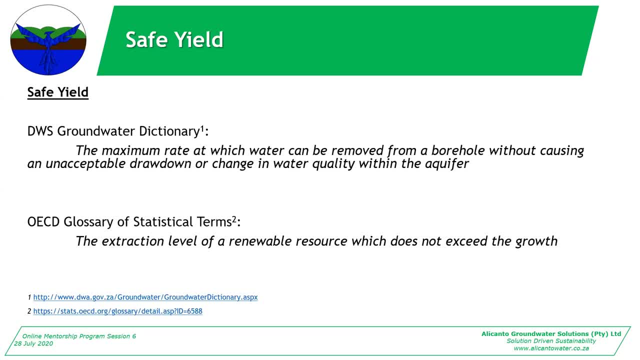 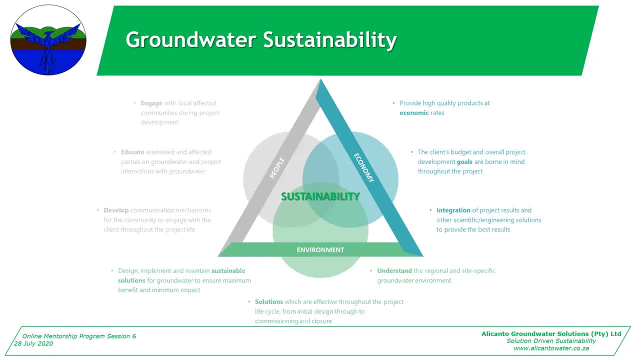 is the same definition but that i don't fully agree with. if you think about sustainability, your sustainability is comprised of your people, the economy and then the environment. so you need to look at the sustainable yield as something that helps the people in the economy. so it's got economic and social benefits but does not negatively impact the, the groundwater. 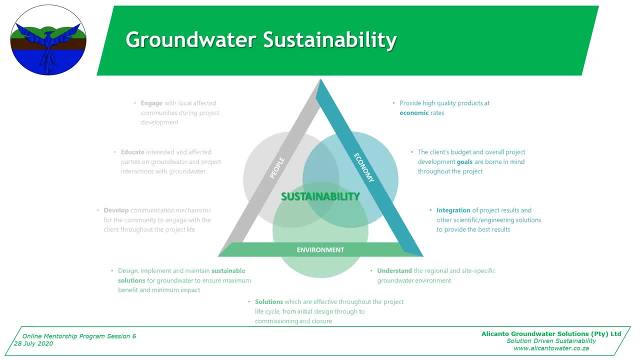 environment or the surrounding environments. does that make sense? the three pillars of sustainability: yes, yes, great. so you've calculated your borehole yield. that's fine, but that may not be the sustainable yield. so that's what we're going to go through now: it's just how to determine if that yield is sustainable for your site. 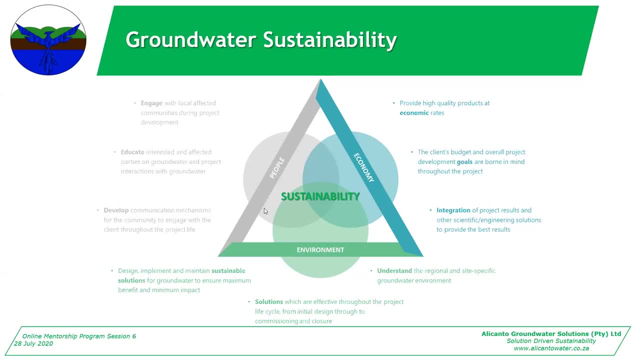 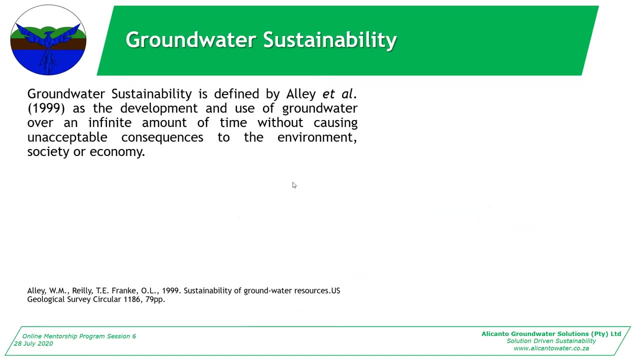 remembering our pillars of sustainability: the social or people, the economy and then the environment. so groundwater sustainability is defined as the development and use of groundwater over an infinite amount of time without causing unacceptable consequences to the environment, society or economy. so the safe yield definition was negative impacts on the aquifer. 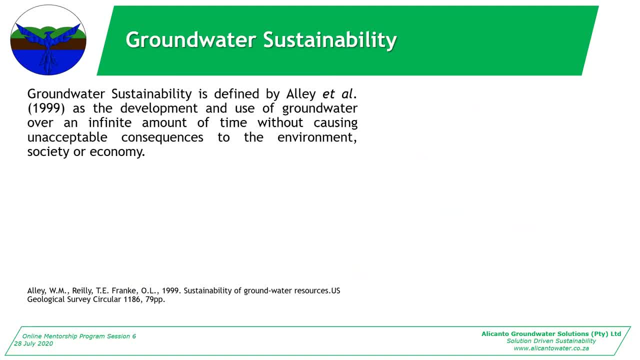 and then the sustainable definition is the both. the environment and the sustainable definition is not the single-use, and sustainable definition is that the solution is sustainable, whereas the sustainable definition is the aquifer, which is part of the environment, the rest of the environment and then society and the economy as well. 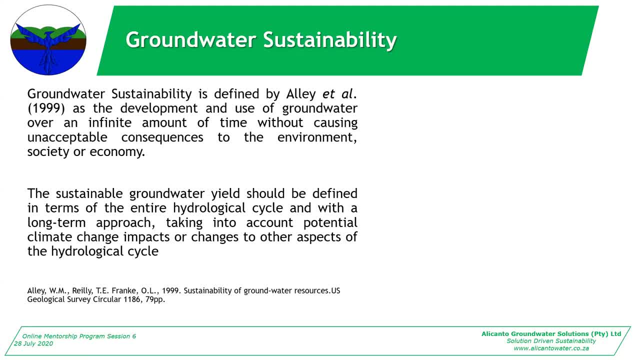 so i, in terms of the sustainable yield, would you really like- well, not make sense, but like, is it really like a good idea, in inverted commas, to really say that it's a sustainable yield because they're talking about an infinite amount of time? but like, really, is really that possible? is that really possible? because sometimes you can have a. 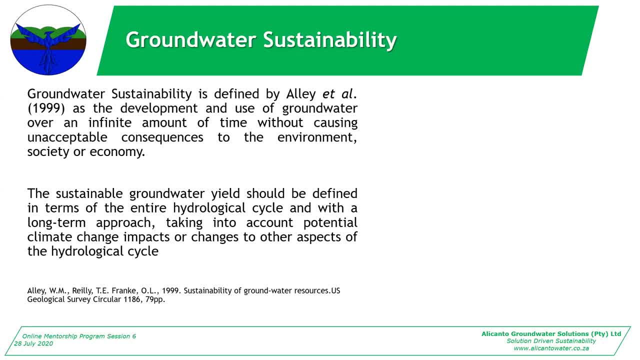 and then your neighbor decides to have a ball and then now it affects your yield and then the sustainable yields that you initially thought was sustainable is not sustainable anymore, because the neighbor now decides to do their own thing. like: does really really sustainable yield exist or is it sustainable given the conditions that we have at this moment, today? now like, 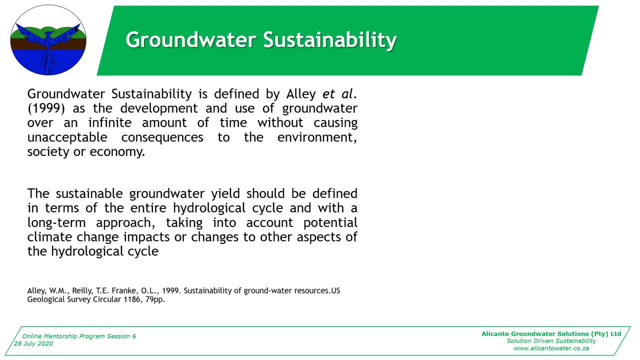 exactly, um, it's like any scientific study or scientific um finding if conditions change. you know it's like most physics experiments and stuff exists in a vacuum. um yeah, sustainable yield, but you know i understand what you're saying about the neighbor. you know if my car can do naught to 106 seconds, but then someone rides into me and knocks off one of my wheels. 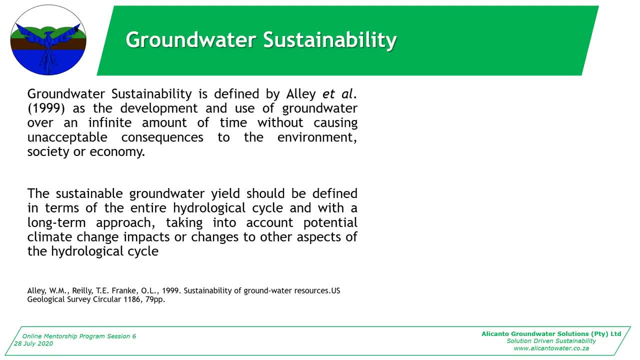 that doesn't mean my car can't do naught to 106 seconds. it means my car is broken. you know what i mean so with sustainable. that's why we do the extrapolation time on fc and remember your pumps have a life cycle. your pumps last 10 to 15 years. your borehole itself has a lifespan of 10 to 15 years. 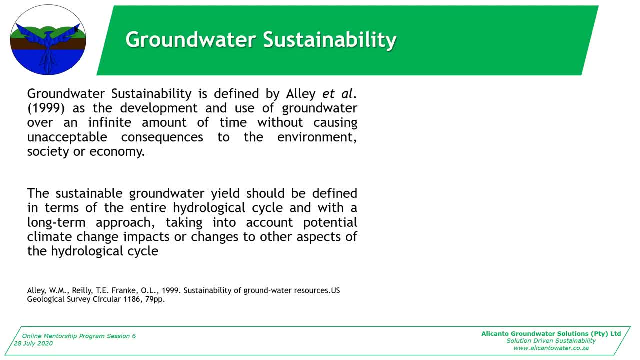 so the infinite time is just a. it's a choice of wording, it's in theory that this should be sustainable forever to make it sustainable, and you know that that's the whole sort of argument, with sustainability as a concept, never mind groundwood of sustainability. you know that's um green electricity and that's an argument that comes. 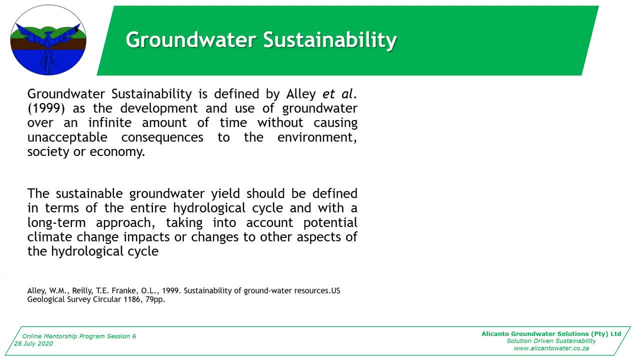 up. is that what happens if? and you can look at what ifs until the sun goes down. but we, we do need to sort of move forward and do the best we can with what we have. okay, thank you. okay, so the sustainable groundwater yield should be defined in terms of the entire. 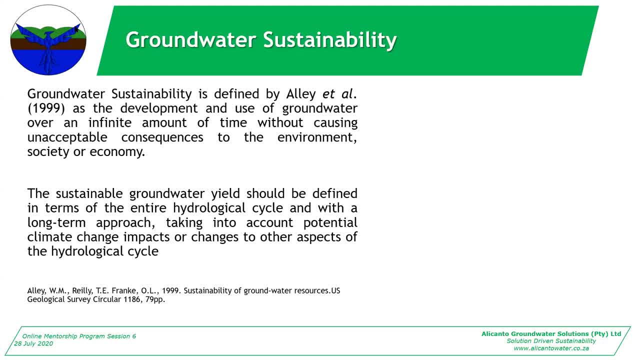 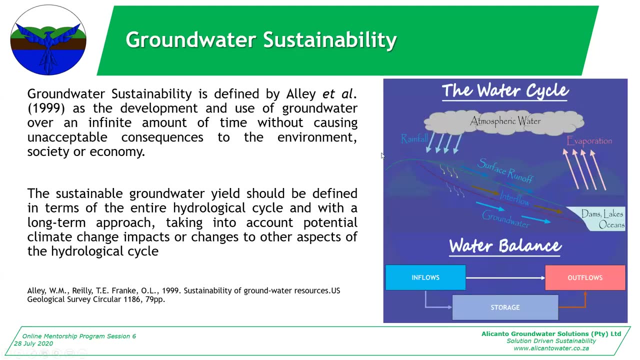 hydrological cycle and with a long-term approach, taking into account potential climate change impacts or changes to other aspects of the hydrological cycle. so that's if your rivers dry up or if the wetlands increase or the rivers flood, etc. so you want to look at your entire water cycle and then the water balance. 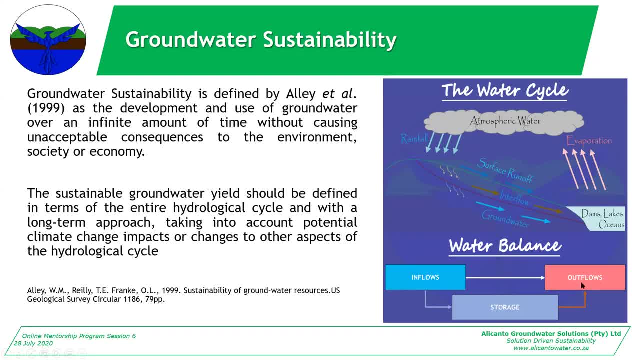 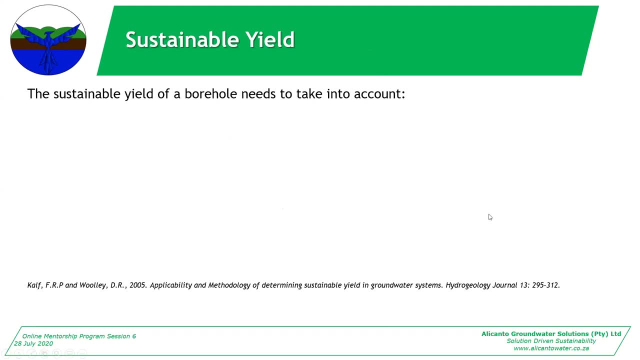 is where inflows and outflows. in a steady state, inflow equals outflows and then typically, your inflows and your change of storage is equal to your outflows. that's the water balance. now the sustainable yield of a borehole needs to take into account, according to kalf and woolly. 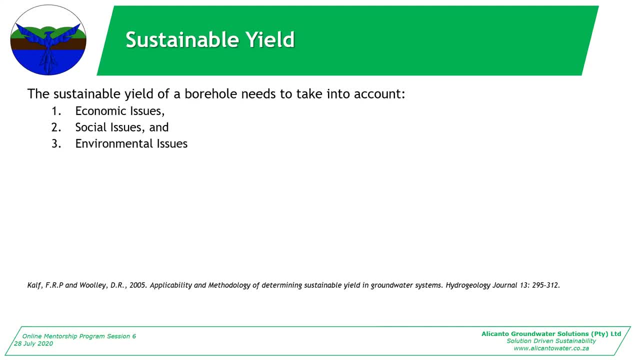 economic issues, social issues and environmental issues. that's again your three pillars of sustainability in a groundwater regime: the groundwater extraction regime measured over a specified plan time frame that allows acceptable levels of stress and protects dependent economic, social and environmental values. if you cannot suggest you read this paper, if you can get hold of it and it. 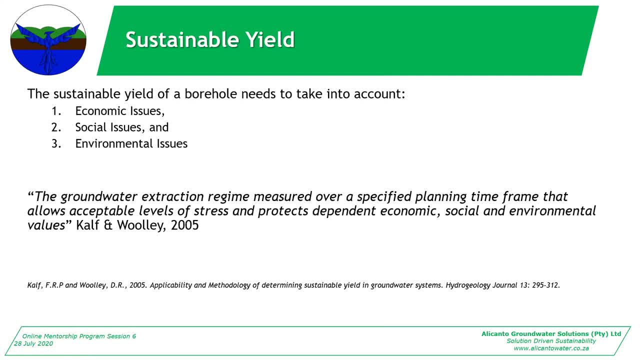 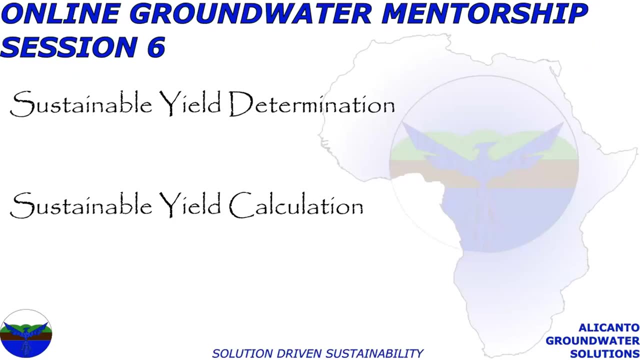 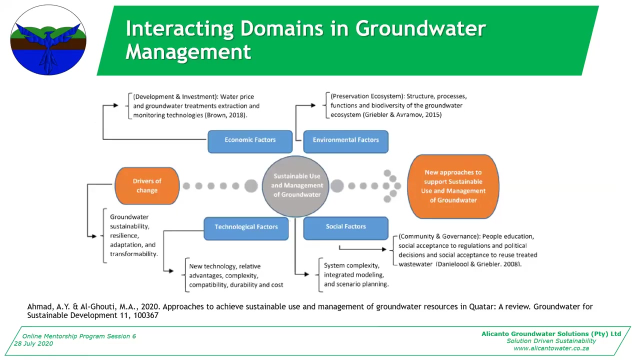 goes through the concepts of sustainable groundwater development quite nicely and it's written in the Australian environment which is fairly similar to the South African one. you know, geologically and climate wise is. now we'll go through how to actually do the sustainable yield calculation now that we've done the sort of definitions, and this is a really nice graphic of all the 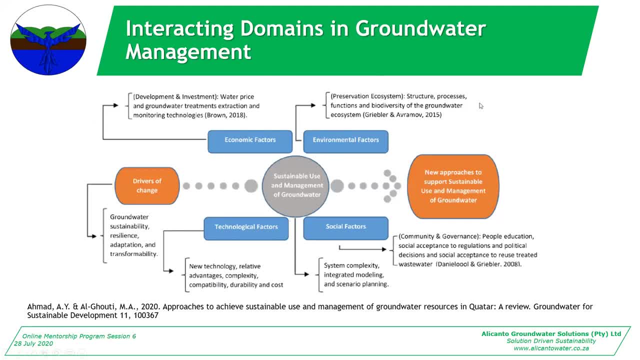 different factors that influence your sustainable groundwater management. so you've got your drivers of change, which is your sustainability of groundwater, the resilience to climate change, the adaption and transmission transform ability of the groundwater resource, and then technological factors: is the new pumps that are available, is the new treatments that are available, that make things accessible that weren't. 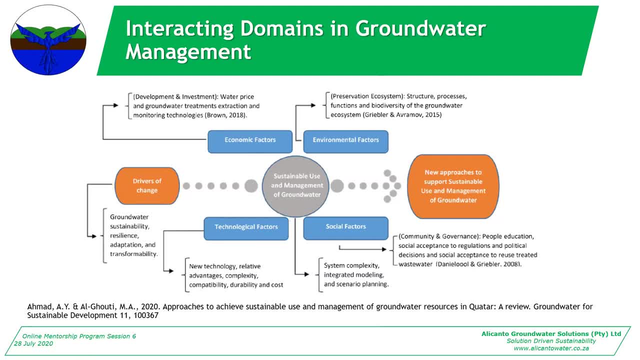 accessible before? how complex are they? how durable are they? how costly are they? environmental factors, such as you know the environmental factors such as protecting your ecosystem, biodiversity of the area. economic factors, obviously, if you're gonna have to charge ten dollars per liter of water to earn some money, if 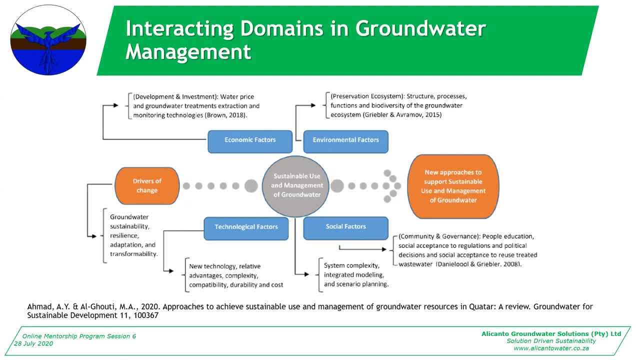 you're selling the water, then it's not economic- people aren't gonna pay that, not now anyway, but economic takes. it takes a big part of water supply and social factors. how complicated is the system? but very short-term, accomplished over time. othernovation ijk, So A lot of African cultures, the guys like in East Africa and in Central Africa the guys. 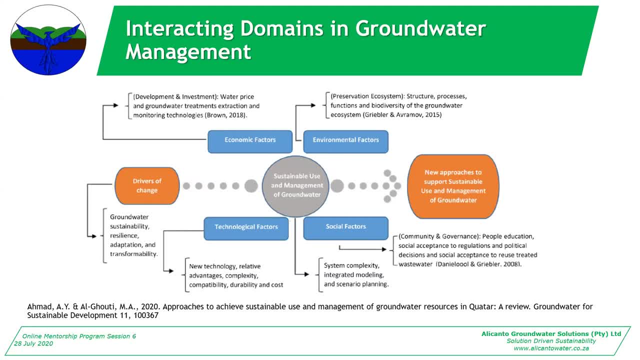 don't trust groundwater. They don't want water from a borehole. That's not sure if anybody's encountered that in South Africa or anywhere that they've worked, but I know in Tanzania they weren't keen on a borehole at all, they wanted river water and that was it. 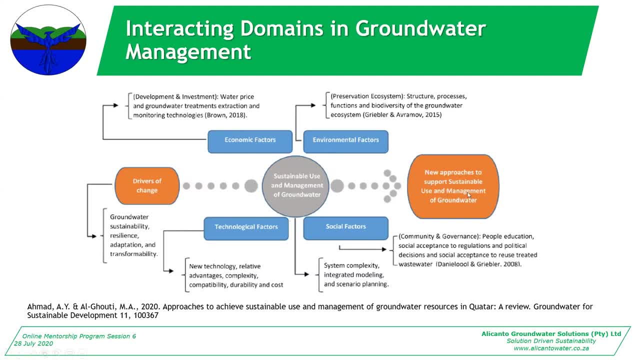 don't want a borehole, don't drill a borehole. and then from all of these factors, you're going to get new approaches to support, support your sustainable use and management of groundwater. and again, if you can, I'd suggest you get this paper, because it's quite an interesting paper, because 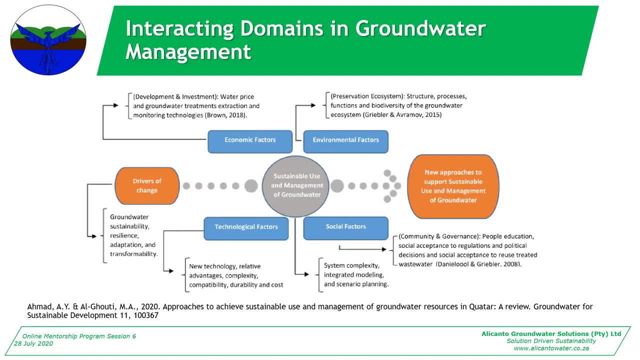 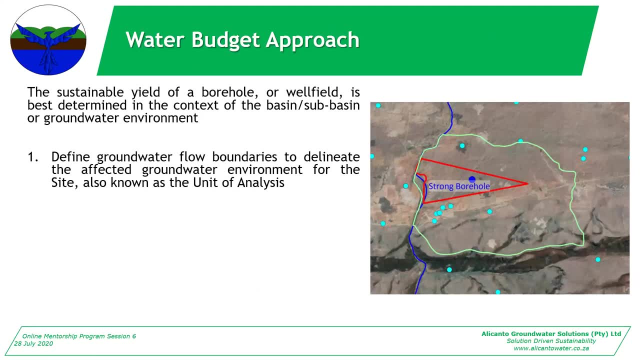 Qatar is a semi-arid to arid environment, a little bit drier than us, but quite interesting nonetheless. okay, so the water budget approach that I typically use in my water use license reports. you can also call this groundwater reserve determination. do you guys still learn the the GRDM method in varsity? I didn't. 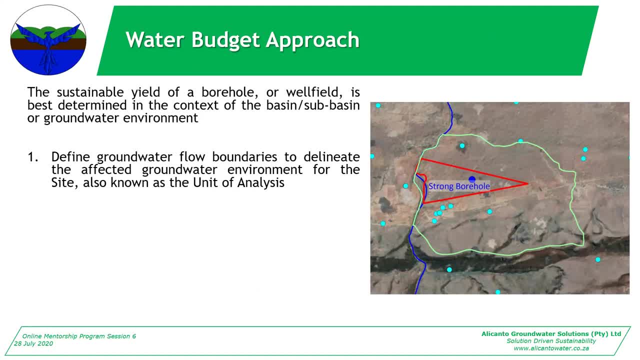 I don't know what it is. what is that groundwater? is the groundwater resource directed measures? well, I'm still in varsity, so maybe it's still coming. I don't know. okay, no, I don't know it. okay, Lizelle, do you guys do it? uh, yes, I think we did, I just can't recall. 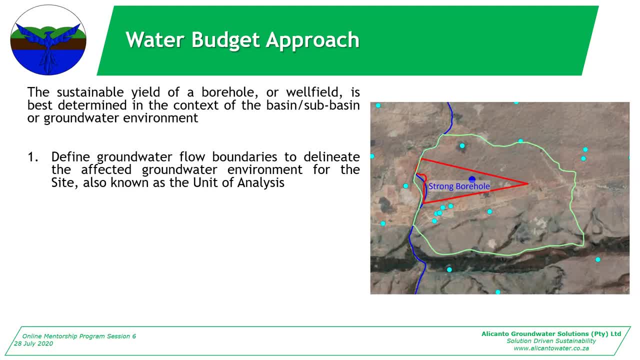 okay, Rachel, I haven't heard of it either. really, Ricky, doesn't make you do it. no, I can't. yeah, okay, now I'll go through it quickly. um, yeah, this is also the water budget approach. this just shows you that your yield is sustainable or not in the long term. can your aquifer system in your 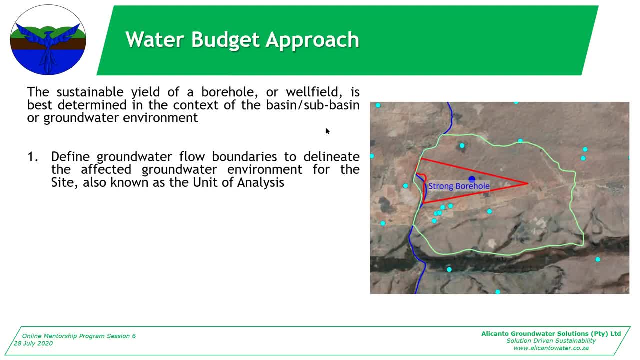 groundwater environment sustain your calculated borehole yield. so the way we do that is we do it in the context of a basin or a sub basin or in your groundwater environment, so that we call our unit of analysis. so these are boundaries to my groundwater flow, so I've got a perennial river here it's. 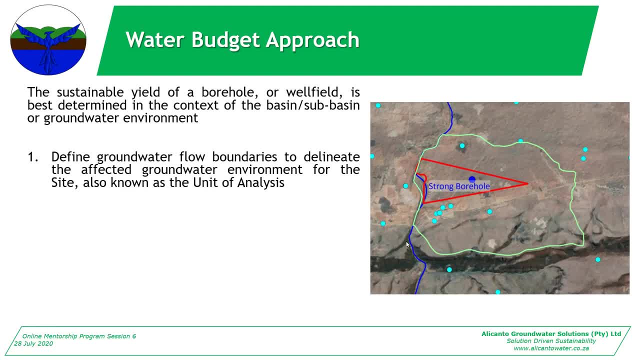 like your model boundaries, which we'll go through on next week or the week after with the modeling section, so groundwater is likely on the site to flow into the river and then into the river. so I've got a boundary to groundwater flow there and here as well because of a river, and then here is just. 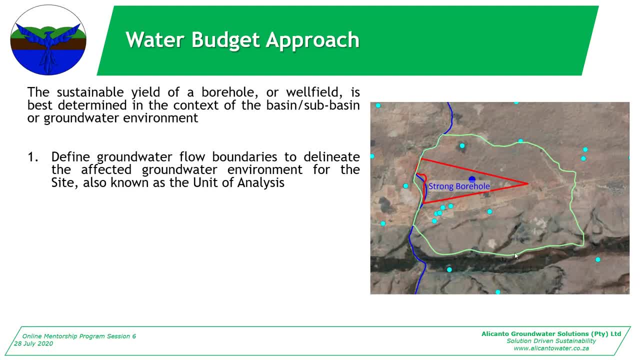 a topographic break. groundwater is not going to flow up the yield and down the hill again, so there's a break. the groundwater will flow down into my site chair, and here is a quaternary catchment boundary which I assumed was representative of groundwater flow as well. okay, so you choose your. 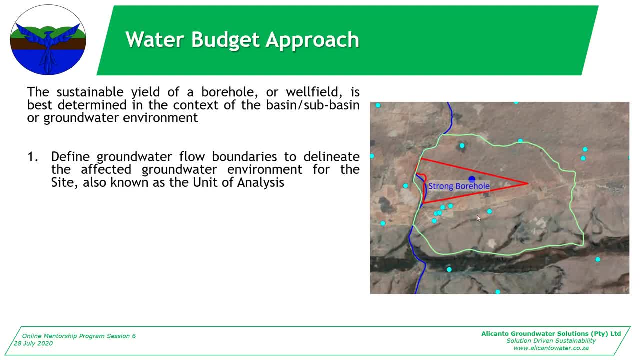 boundary and the boundary will flow down into the river. so that's the boundary model boundaries or your catchment boundaries for the site. this is my environment, where groundwater is going to come into my borehole. that was called strong borehole, this dark blue dot. does that make sense to everybody? yes, cool. 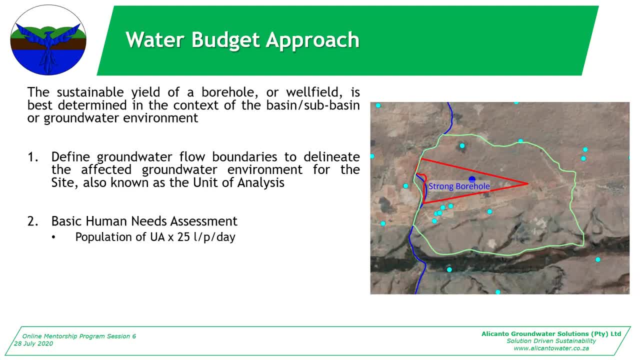 okay, next step: you calculate your basic human needs assessment, which you get from your census databases, and you look at it. yeah, how many people are within my unit of analysis? you take that population number multiplied by the 25 liters per person per day, which is- I think it's the UN or who- bare minimum. 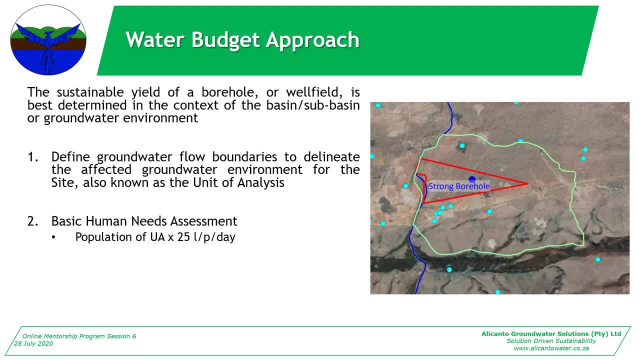 for people. so if I've got a hundred people it'll be 2,500 liters per person per day. then you calculate that need per annum, you and you do ground water contribution to base flow. you can do that by hydrograph separation if you have hydrographs, which is your river flow rates over time or 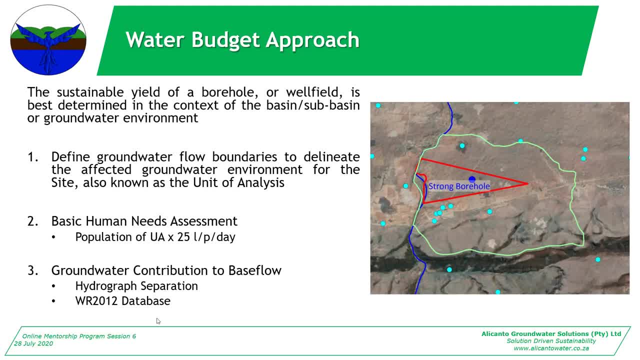 you can just get it from the WR 2012 or G ODM databases, where it'll tell you for this catchment. there's a question? okay, Lee cleared. how do you determine the boundaries? your boundaries are the boundaries to groundwater flow, so we'll go through it. 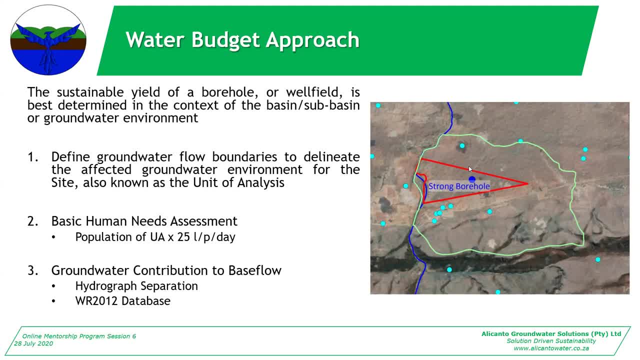 in detail with the modeling section. but it's where, like, groundwater won't flow across this perennial river in this environment, so that's a boundary. then it won't flow across this channel here, so that's a boundary. then here is a topographic divide, because groundwater can't flow uphill and then downhill and 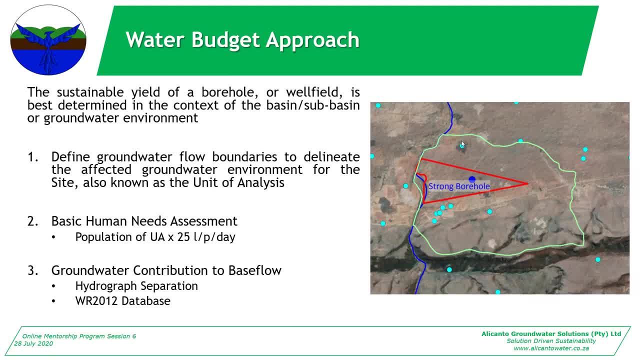 then prior down and then flat. it will be mean going right down to the top and down to the top editorial σThis is to determine how these haveścipies will fall. for example, a pipe like this parallel into an echo-type of turn signal. 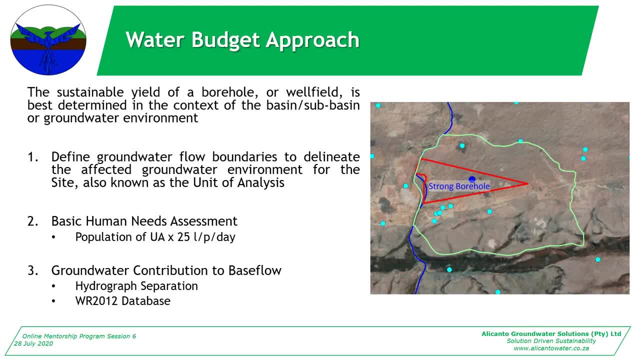 among those boundary or without this turn signal. that means he felt the explain. I do get the boundary on the river boundary and the one at the bottom, but it's the other two that I don't get. how you would define those boundaries, or would we go through? 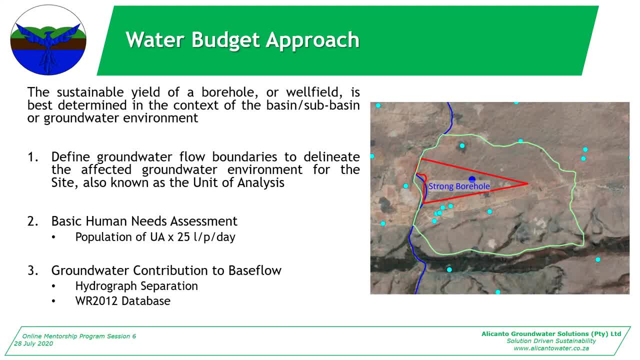 that when we doing the modeling section it's environment specific. you know, on this one we had a non-perennial channel here and a geological contact, so you've got like a hard quartzite here and then a sandstone here. so it's unlikely that huge amounts of water are going to go. 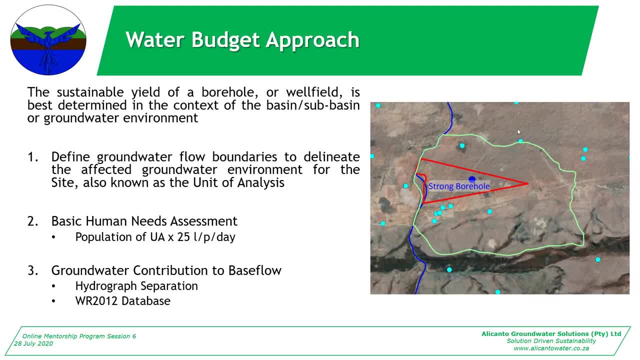 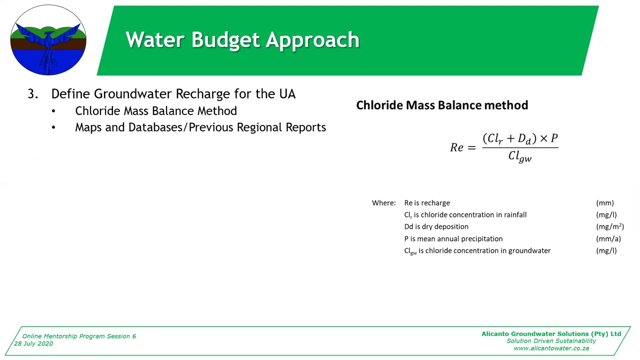 through into the quartzite from the sandstone. all right, it's. it's not specific, but we'll go through it with the modeling session. all right, thank you. so we've got unit of analysis. then we do our basic human needs assessment and the groundwater base flow contribution and then we have to define our ground with a recharge for the unit of. 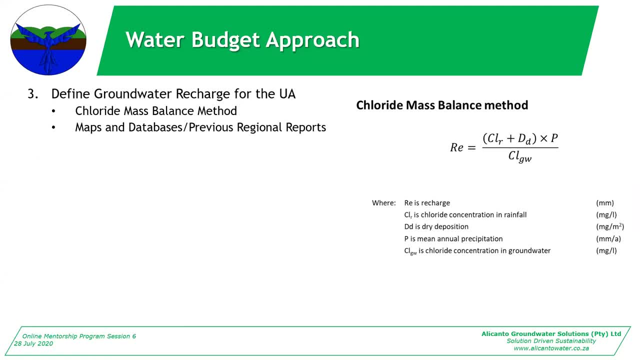 analysis. you do this by the chloride mass balance method, if you have it, or you look at your maps, your factor map databases. you know any regional databases, your soil maps, ground with the harvest potential or previous reports for the region or near to the site, the more data. 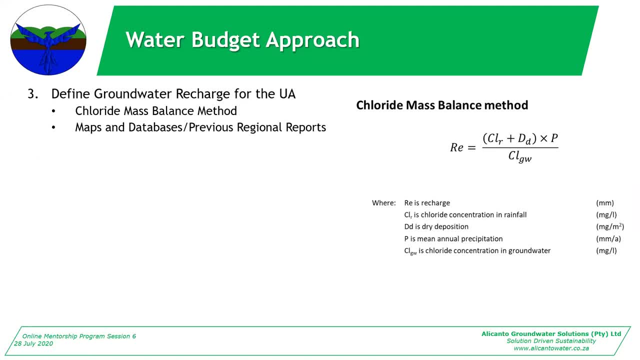 you have the better. if you can get a hundred different recharge points and take an average, that's great. yeah, it'll help you defend your, your recharge value that you assign. there's just the recharge method or the chloride mass balance method for recharge calculation. then Existing abstraction is also important. 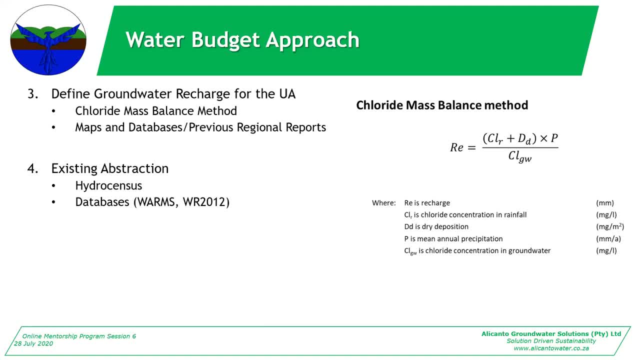 That you'll get from your hydrosenses or from the regional databases, such as Worms or the WR2012 database. That's: who's pumping out of this aquifer already? Is my neighbor pumping? That relates back to the question we had earlier. 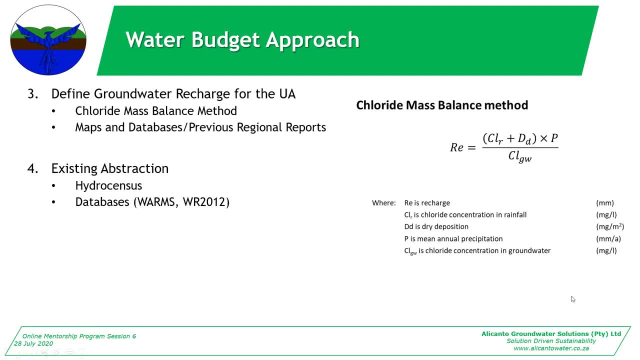 about sustainable yield and neighbors, etc. When you do the water budget, you take into account the existing abstraction. If your neighbor wants to drill a ball, he should take into account your existing abstraction. Then you have your proposed abstraction, which is your calculated borehole yield. 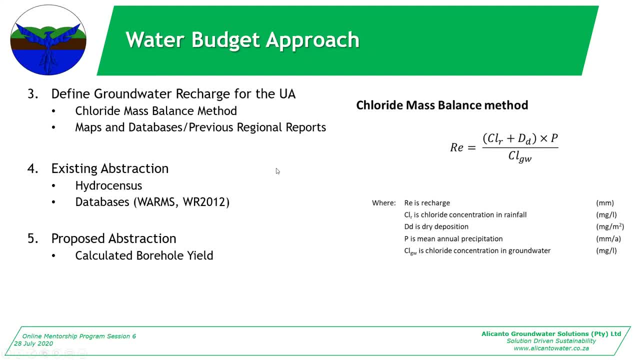 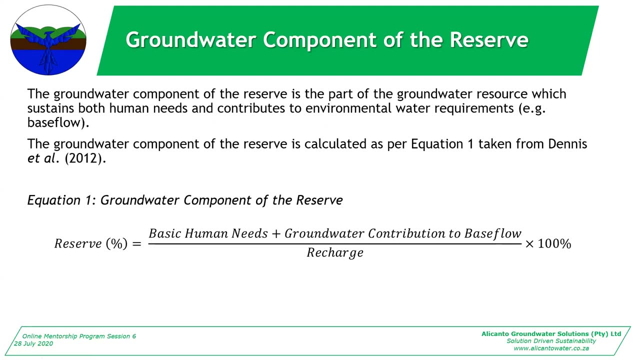 Is everybody with me in terms of what we need to get together for our water budget? Yes, Pretty straightforward. Then we calculate the groundwater components of the reserve, which is the part of the groundwater resource which sustains both human needs and contributes to environmental water requirements. 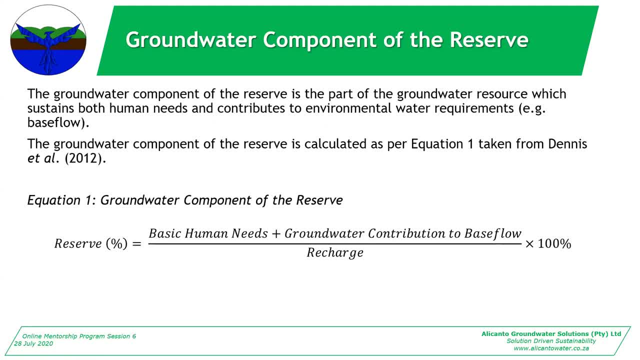 such as your base flow, Your base flow. that's why the base flow calculations are important. The base flow could be to a river or to a wetland or to any kind of surface water feature, If groundwater feeds that feature in the dry season. 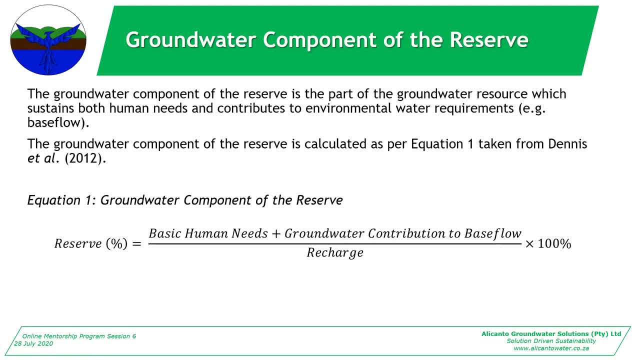 or whenever that is base flow. The groundwater component of the reserve is calculated by taking your basic human needs plus the contribution to base flow and you divide that by my total recharge. That'll give you a percentage. That is the percentage that you cannot touch. 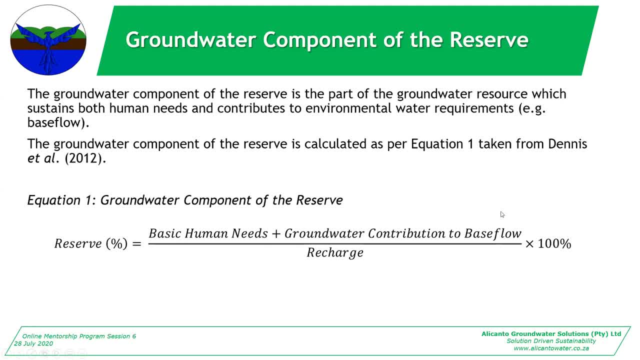 You need to have groundwater to meet basic human needs and you need to have groundwater that doesn't take away from the existing environment. That's your base flow, You know, because realistically, groundwater doesn't contribute to the environment other than base flow. Does that make sense to everybody? 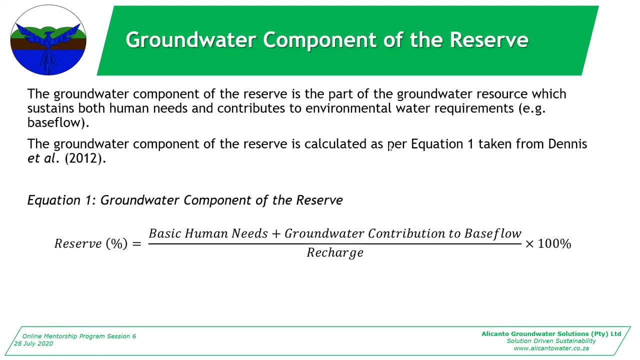 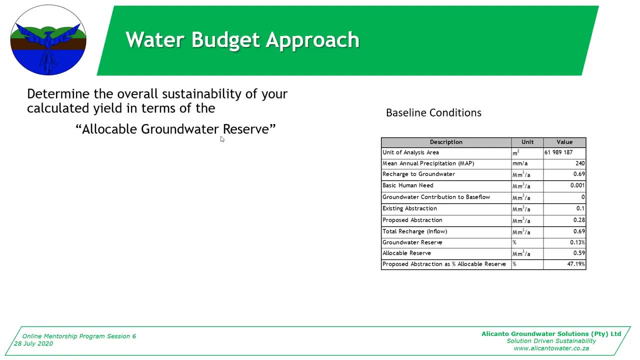 Yes, Matthew, it does Cool. So then you determine the overall sustainability of your calculated yield in terms of the allocable groundwater reserve. So I've got my area in meters squared of my unit of analysis, My mean annual precipitation, And I use that those two 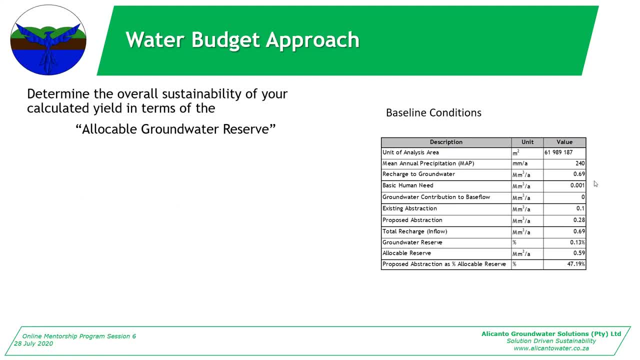 to calculate my volume of recharge per annum. We use the mega cubic meters per annum, So that's million cubes per annum. So I've got 0.69 recharge. My basic human need was 0.001.. Groundwater contribution was zero. 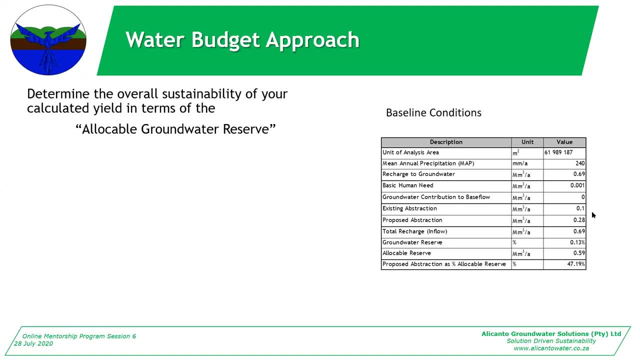 because that's a losing river on this side, So the river feeds groundwater, not the other way. Existing abstraction in the catchment was 0.1, which was actually- it was my client's other borehole- And then the proposed abstraction was 0.28. 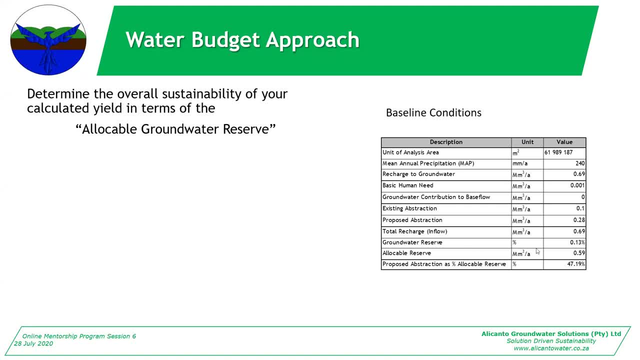 mega cubes per annum. So then I calculate my groundwater reserve. So my total recharge is 0.69. And my groundwater reserve was 0.13 of that 0.69.. So that is basically 0.69.. Basic human need plus my contribution to base flow. 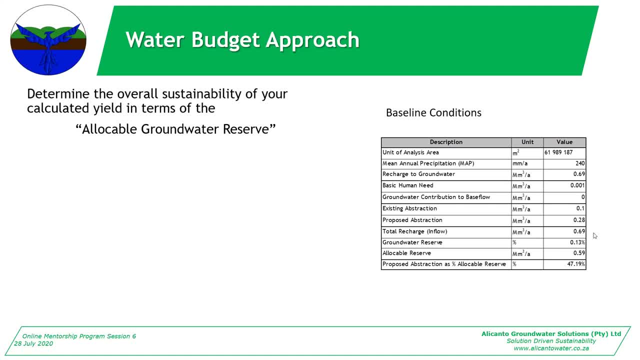 Gives me 0.13.. So that is what I cannot touch out of that recharge component, which leaves me with an allocable reserve of 0.59.. Does that make sense to everybody? Yep, Cool. So then what I do is I take my proposed abstraction rate. 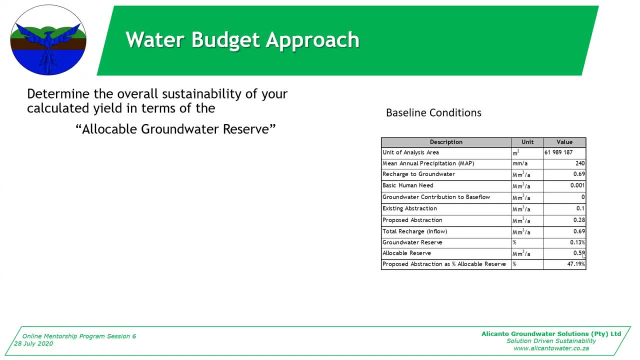 that I've calculated and divided by the allocable reserve and I can see it's less than 50% of that allocable reserve. so do you see that means that my calculated borehole rate is sustainable, because I'm not getting up to the 90% of. 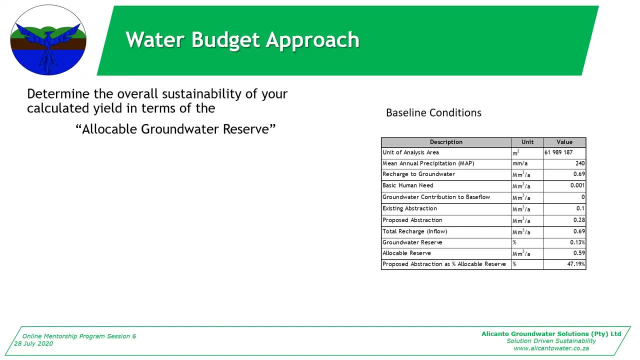 what's left over like there's still more than enough water to meet the environmental requirements and the social requirements if they increase. so there's my sustainable yield. I've proved that my borehole calculated yield is actually sustainable in the context of the site and you can use this to run. 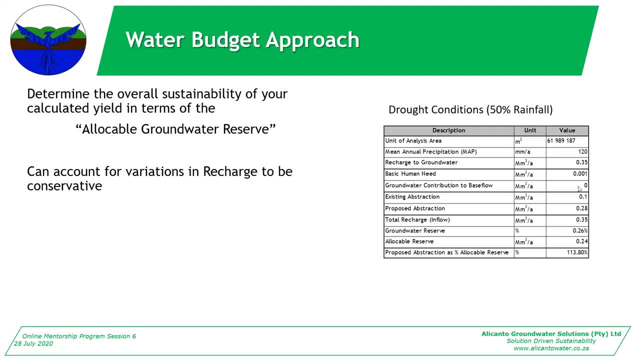 different scenarios. so, for example, if I had to half the rainfall, which means I'll half my recharged groundwater, then my calculated yield becomes a hundred and thirteen percent of the allocable reserve, which means that my borehole rate is actually more than 50% of what's left over. 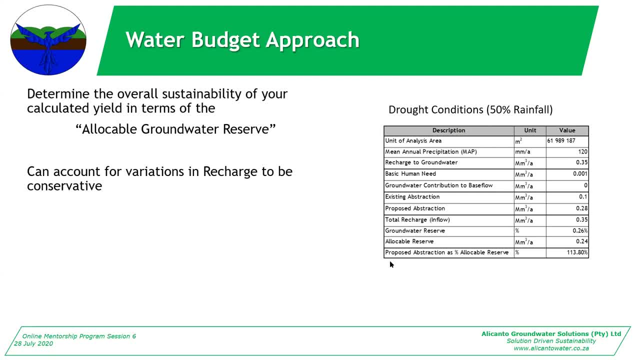 which means it's not sustainable. so therefore, if it's in a drought prone area or if your climate change data suggests it's going to go into a drought, you need to adjust your calculated yield, but to 75%, so 0.21 instead of 0.28 to be. 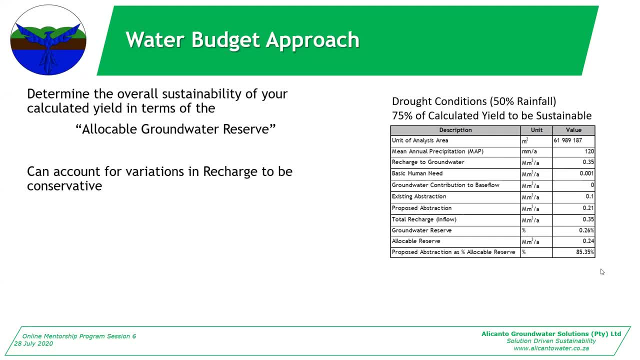 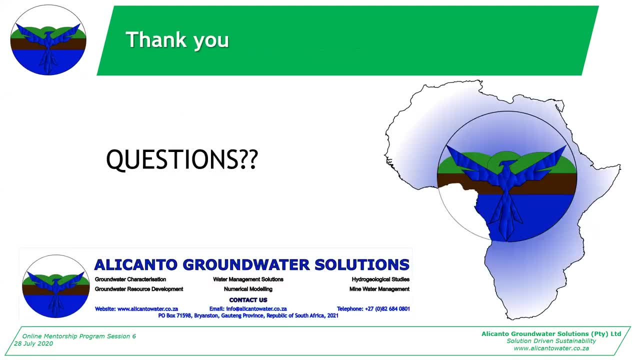 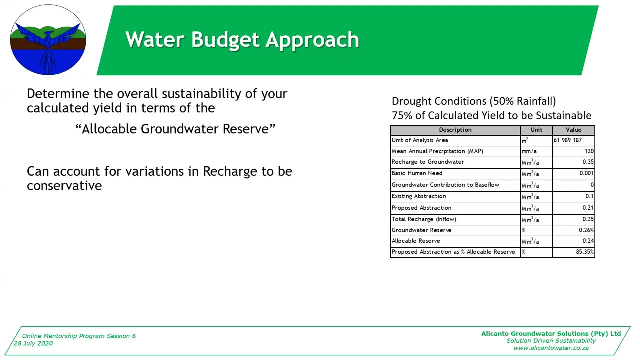 sustainable to be less than 90% of your allocable reserve. yeah, so you see it. that's a fairly straightforward concept to calculate your budget and say: this is what's important for the environment. this is what I want to take out of it. yeah, is it sustainable or not? everybody agree that it's simple. 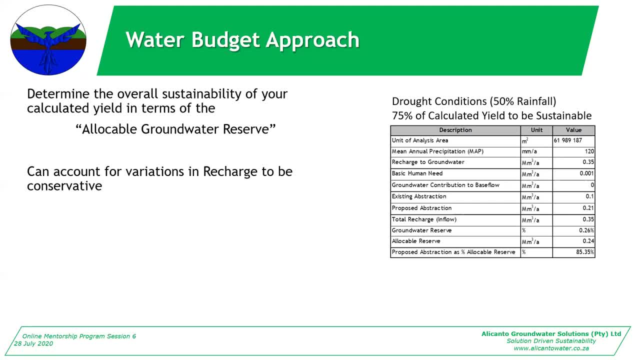 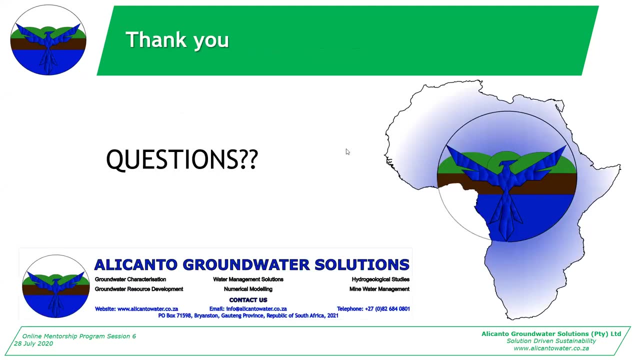 or is it confusing? it makes sense. so, yeah, that's the end of it. so are there any questions about sustainable yields, safe yields, FC? what we've gone through today, Matthew, that that FC program seems very complicated. like it seems very complicated, but one day I'll download it and like try to figure out how to do it. 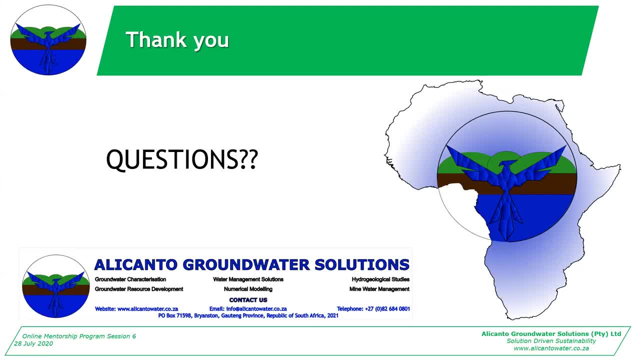 in a week. I'll do it in a couple days and then we'll talk about it in the next two weeks. so the part of the 비유 is it's really not that complicated if you are somebody who's always trying to get started on your own job. 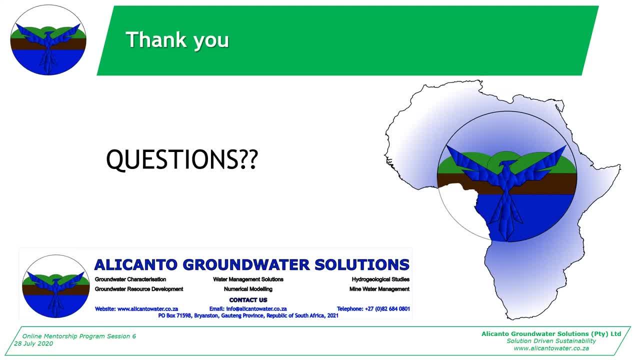 then you can just come out of it right away in your next few weeks. but a lot of it is just a little bit of it and end up being a little bit more complex, so you really should have time to go through it. you can probably do it on Friday. 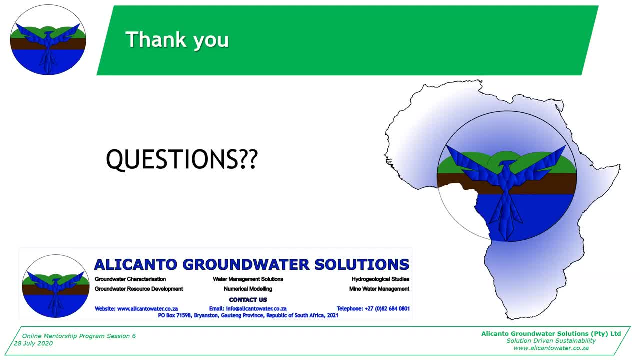 or Saturday. the faster the better it will be. so if you're trying to get started on a plan, you can actually start with this one. it's more complicated than you might think if you go through it later. if you're trying to get started on your own job. 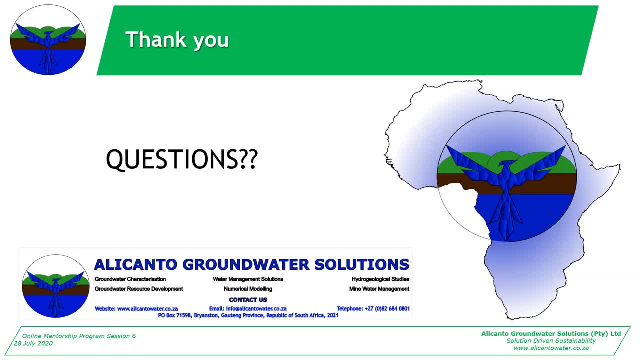 but that's really it's. it depends: if you want to do all of the methods, it's complicated, but if you want to do more of it, you can do it. anyway complicated, but if you just want to do the, the cooper, jacob and the basic fc, it's not that bad. 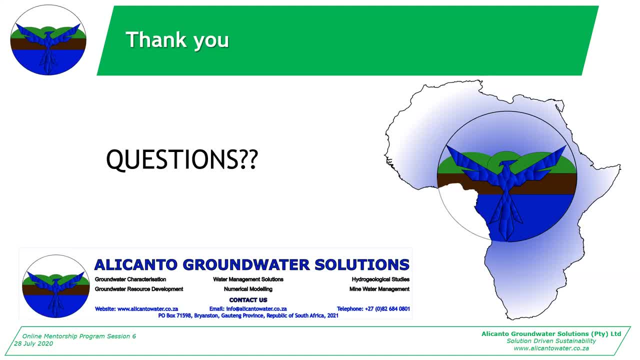 yeah, the, the cooper jacob, that i understand in the basic i i understand, but the rest i did not hear what you said. i did not understand what you said. how do you mean on the excel, on the excel spreadsheet, um there was, i don't know which, which, um which data set. 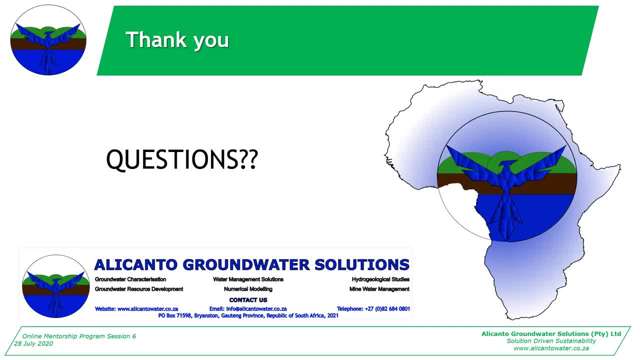 you were working with what you were calculating. they- i think it was the interception or something like that, or inflection, or yeah, the inflection point, yeah, yes, okay, now i think let's go through it with the other aquifer testing on thursday and then you'll see it'll make a little bit more sense. okay, thank you, but don't stress. 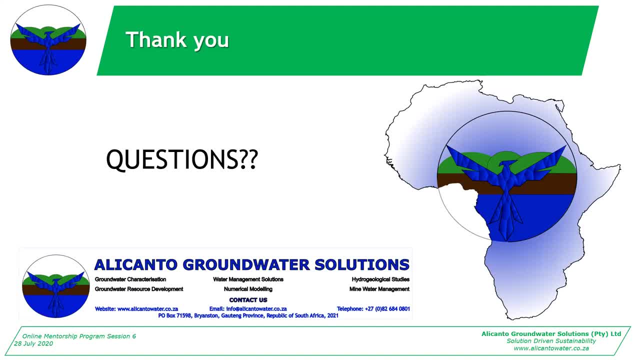 about it, don't be scared of it. yeah, we've got control z undo, it's not an issue. okay, thank you, cool. any other questions? um hi, matthew, i just wanted to ask if the slides will be available, just for me to look over everything again and get those papers. 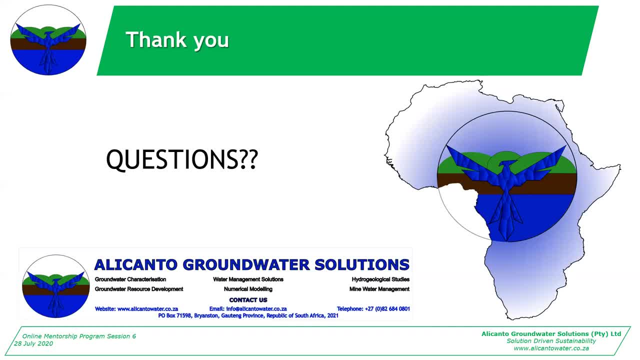 yep, definitely, um, i'll upload it to the website um tomorrow and then, um, you can just go to the company website and go to the download section. okay, um, all of the the slides are there, and then all of the previous slides are also up. oh great, thanks so much. no, i mean if there's any questions. 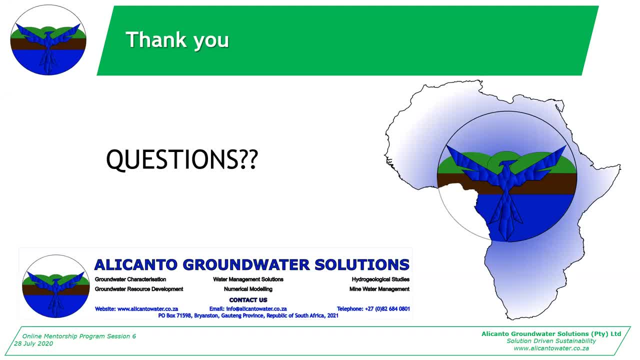 just send an email through and uh, yeah, no worries, we'll go from there. thanks, cool, any questions on sustainable yields? and that, stephen? no, i just wanted to say thanks, matthew, that was great today. thanks a lot. no, thanks, guys. any questions? um, no, this one has. yeah well, it kind of doesn't have anything. 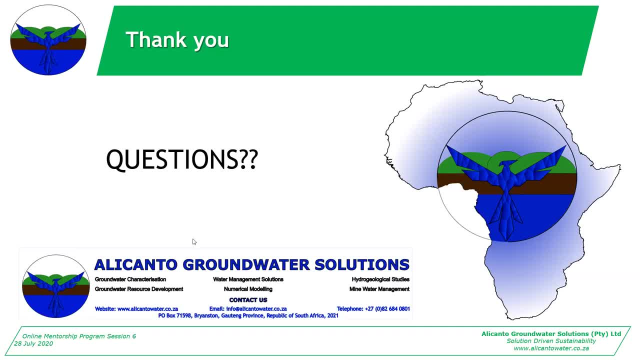 to do with today, but even jay the whole process of um from like the first, first, from the beginning, up until the end, like in terms of producing the report, in terms of doing the pumping test and and whatnot, and whatnot. how long generally does it take you to do like the entire thing for you? 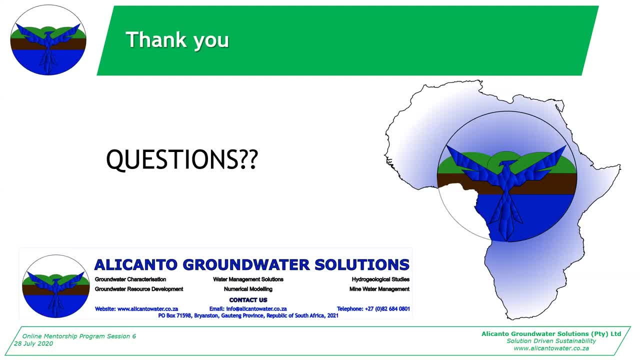 to actually know everything about that boho and the yield and the pump that you need to get, and, yeah, until, like, until let's say somebody, yeah, people will know how to do it because they're fun for them and they really understand the same thing, you know. but, yeah, i couldn't be more than a reminder that this is not a 100 year philanthropy, so, yeah, i won't go into it. but, um, yeah, next website will let me drop you some, yeah, and then we'll share the current relationship with the plan and so on. until then, let's talk about some other topics. um, okay, together. okay, so, thank you, jife came from jai today. good, 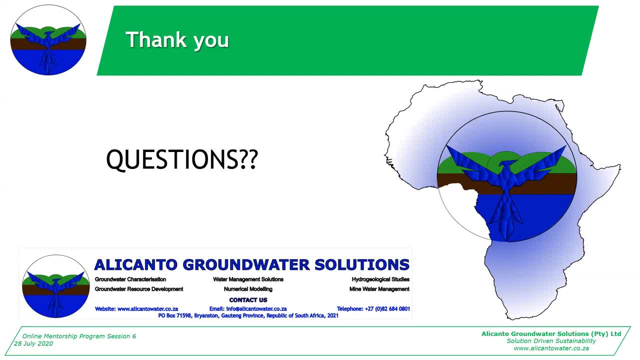 let's say somebody- yeah, people use it for like human consumption, like for everyday basic needs like how, how long generally does it take you? yeah, look, i mean a thumbsack- um, for something that's within 100 kilometers of the office. i would say four to six weeks, um, including about 10 days, 10. working days for the laboratory results, and also it depends on your client. if your client wants you to do one thing at a time, then it can take up to eight to ten weeks, and then if it's a far away site, that obviously takes longer because you've got to drive out to do the geophysics. then you come back to the office and interpret. but maximum you're looking at probably about three months. so 12 weeks, okay, okay, yeah, and minimum you're looking at four weeks, okay, interesting, yeah. look, sometimes projects come together but other times they fall apart. and then when they fall apart, is it on you, like, are you okay? obviously it's on you. there's more. 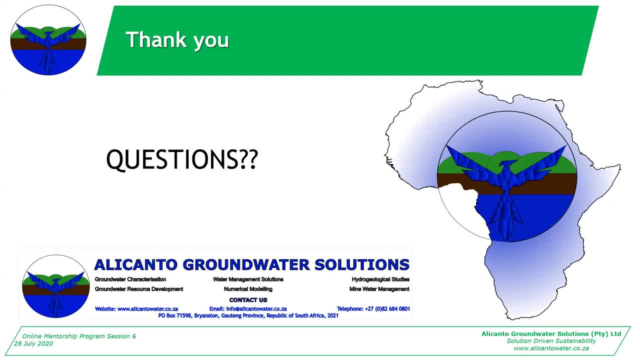 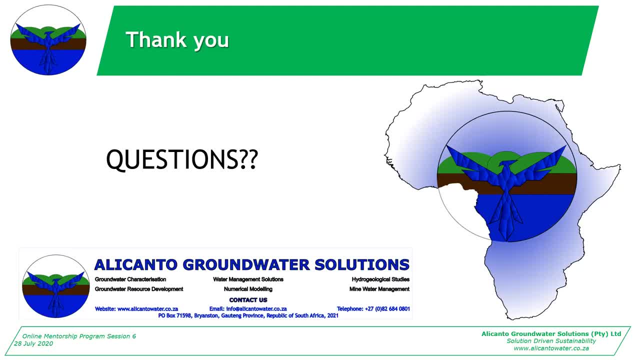 and then the driller will tell you you need to pay for it and the client will say he's not paying for it. and then you're gonna sit there fishing for a drill rod for three weeks. um other times you drill a dry ball. the client doesn't want to pay you, or the client makes you. 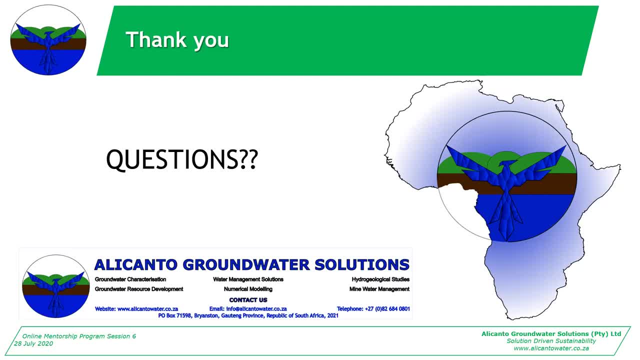 drill another ball and you know that there's so many things that can't go wrong from a personal or a personnel perspective. you know you can have an incident on site and your site gets shut down. you could have it where- i mean, i've had it- where they drilled into dolomites. 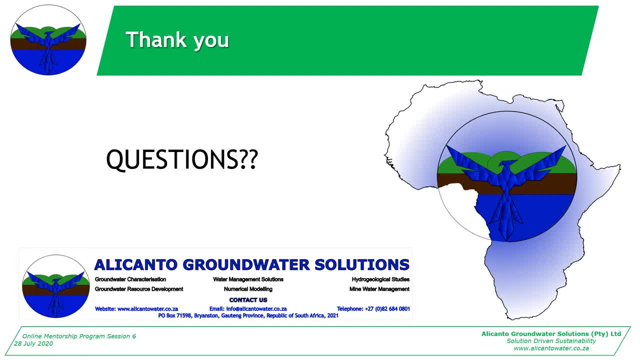 and then the dolomites collapsed on the rod and they lost the hammer, the rods, everything, and the driller spent three weeks trying to get his rods back. yeah, so every every site is different. you've just got to. you know, i've said it before: you've got to manage your liabilities in your contract. you've got to make sure. 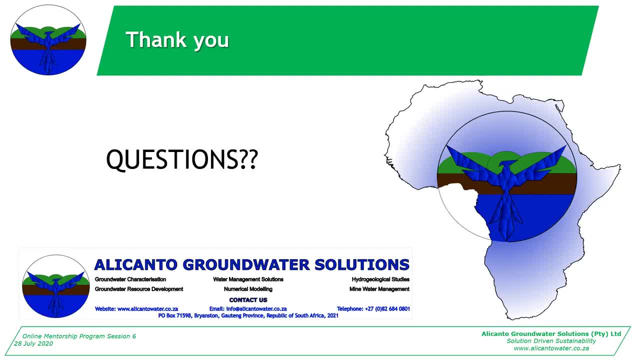 that everybody is responsible for their own part of the world. your driller must look after drillers and drilling equipment and you must look after the site and the clients interests. yeah, thank you, read, read the contracts, because a lot of drillers and the initial proposal they'll say to you you. 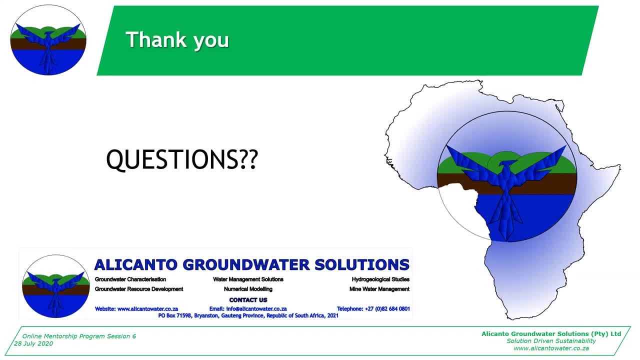 are liable for the equipment that gets lost or damaged. you know, negotiate that and say to them: listen, this is a hard rock environment, so you are going to lose bits. the bits are going to get worn, but I'm not going to pay for a new drilling. but be upfront in your negotiations. okay, yeah, don't let it be a. 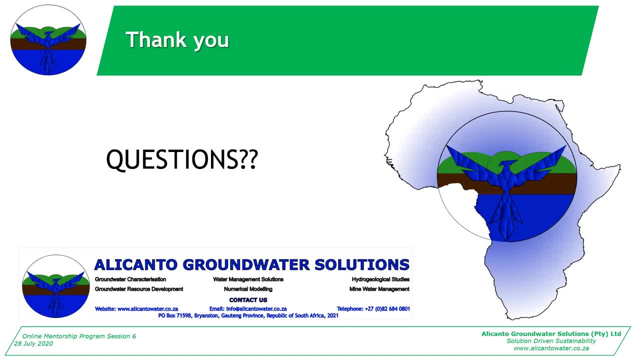 surprise later when there's a couple thousand rand on the line. yeah, cool, cool, Matthew. hmm, I wanna ask how much does the whole thing cost, from the hydro sensors or up to the sustainability and then the reporting part, like the whole project, when including everything, how much like? 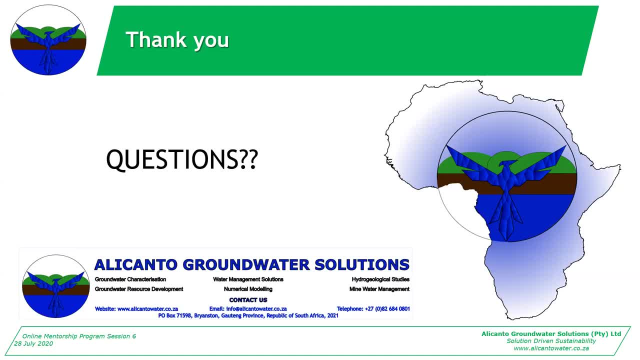 generally does it cost? look, I mean your costs, including drilling, aquifer testing. that costs everything and your pumps. you're looking at anywhere between a hundred and fifty thousand and two hundred and fifty thousand rand for one borehole. let's see if you do everything top of the line. you know you do proper. 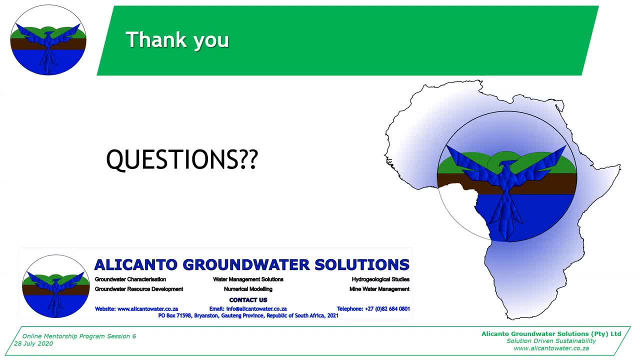 drilling, proper casing, but you can get away with a hundred and twenty thousand, two hundred and fifty thousand rand. okay, your, your main cost is your drilling. I mean, you get drillers that charge anywhere between three hundred and six hundred rand a meter, but if you go into larger diameters you're looking at. 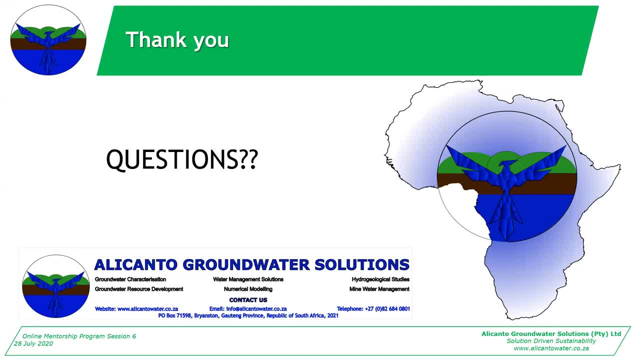 potentially a thousand two thousand two hundred rand a meter drilling cost. okay, anybody else? um, just to comment on on babyliss? um question, actually, we are actually well where I work I will put a department of water first. so we are actually doing a borehole like custom model and it would actually be very helpful if you know. I 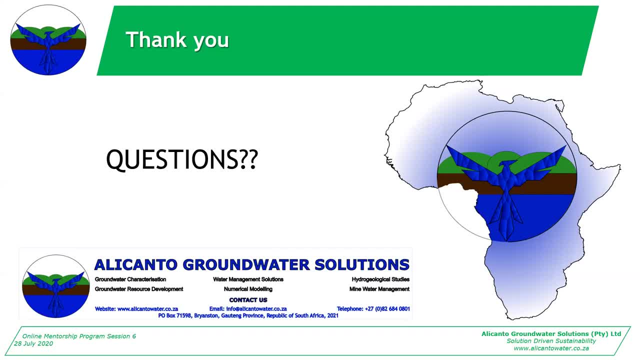 can send some of my stuff to you, Matthew, and then you just like give me an idea of like, because we already have the model but we are like kind of refining it, because the babyliss question of how much actually like a lot of people are scammers- well, not scammers, scammers. but 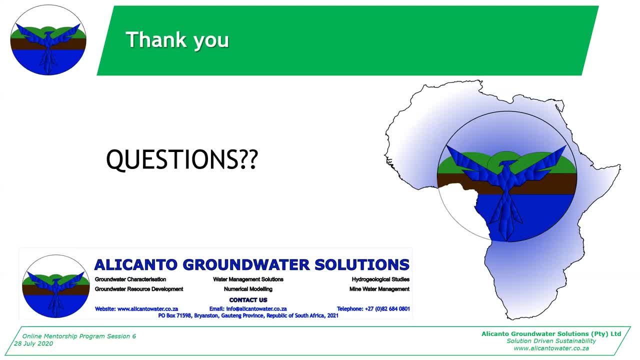 like they. they will scam you. you know they will charge you like millions and millions, especially if they're charging like directly the government. they charge millions and millions when it's not really like that. that that much. so yeah, babyliss question is very important and I'm working on it, so yeah. 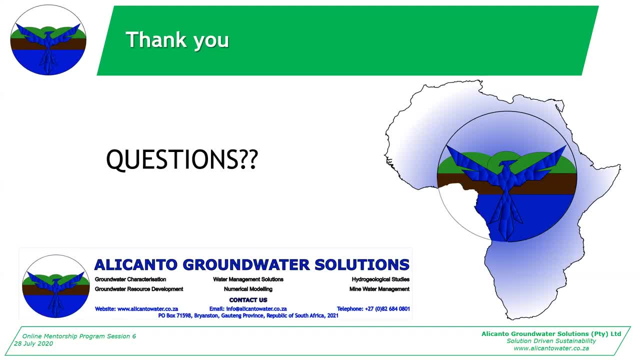 no, that's interesting. yeah, look, if you can share it that'll be great. um, you know, because I I know a lot of. I can't remember what it was for, but it was like a scandal where the drilling contractors were charging like a million Rand a borehole for water affairs. I think I might have been Cape Town with the drought relief. 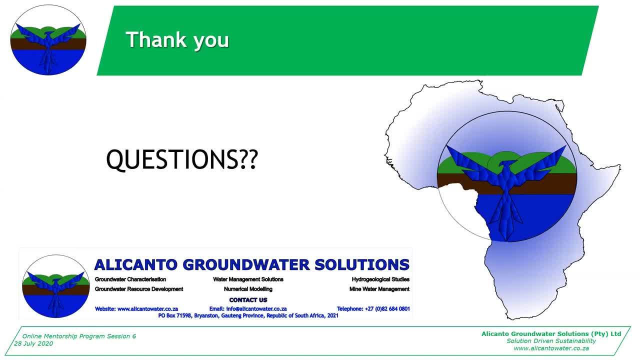 um, you know there was a big thing last year or the year before. yeah, because it's uh, it happens and the thing is also, drillers will charge. like I know the water affairs drillers- I've heard stories about them. I don't think you have a drilling department anymore. 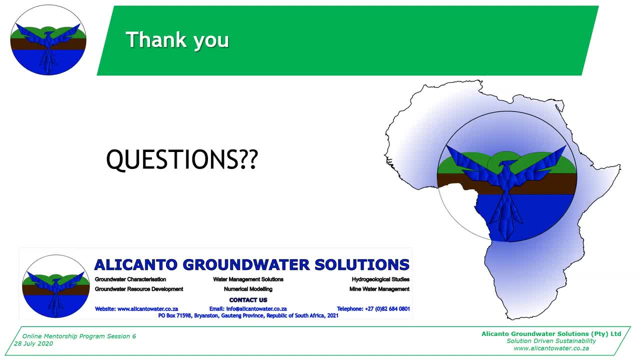 but um, you know, the old guys would tell me stories about because they got paid per day, not per meter, so they would take 20 days to drill one borehole. yeah, so you know, most drillers get charged or get paid per meter, so the more they drill, the 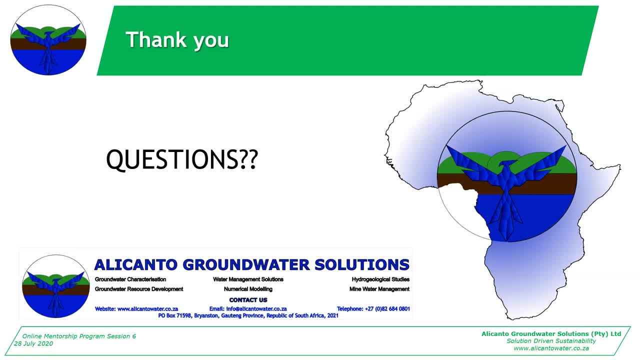 more they get paid. yeah, no, but I'll definitely send my model and then you can check it out and see if it actually makes sense. yeah, thanks, just clear it with your, your bosses, first. oh, yeah, I did okay. yeah, I don't want you guys sharing stuff you're not supposed to. yeah, yeah, I know how that means, but how important. 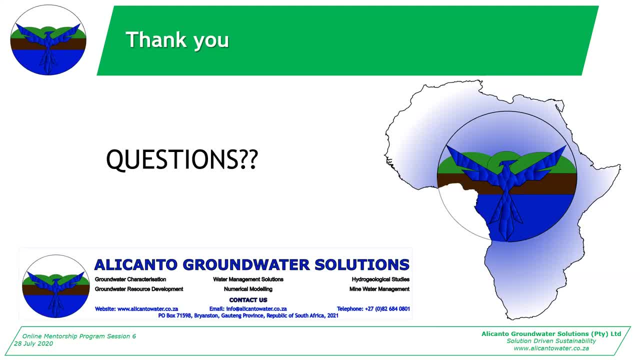 no, but thanks, I appreciate that. uh, I think it'll be nice for the group you know maybe can present it to everyone and explain it a bit. yeah, awesome, thank you. thank you, i'd really also appreciate it great. so, everybody happy we're going to carry on on. thursday again: we'll go. 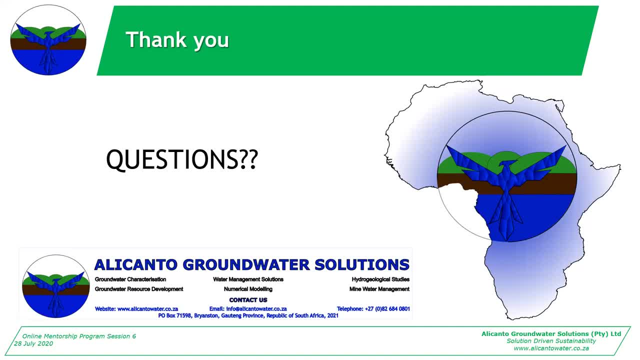 through the task and all that stuff. yes, thanks, awesome, okay, so thank you very much, guys. uh, thanks for joining us, and i hope everybody learned something about the sustainable yield and the groundwater resource development cycle over the past couple days, and we'll pick it up on thursday again. 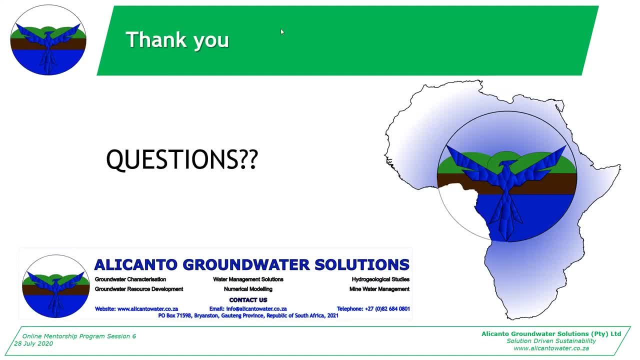 bye, cheers, guys, have a good week.